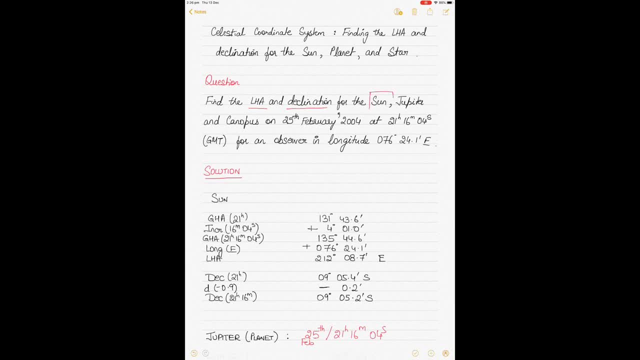 Okay, let's start by focusing first on the sun. The date is 25th of February 2004 and the GMT time is 2100 hours 16 minutes and 4 seconds. Because it's a GMT time, we don't need to apply any correction to it. We can straight away use this time to obtain the values from the nautical almanac, And the longitude given to us is 076 degrees 24.1 minutes east. 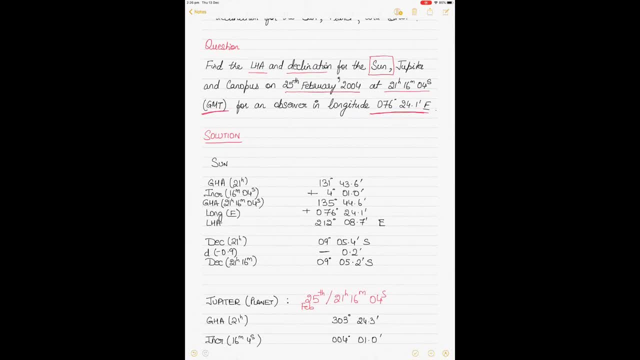 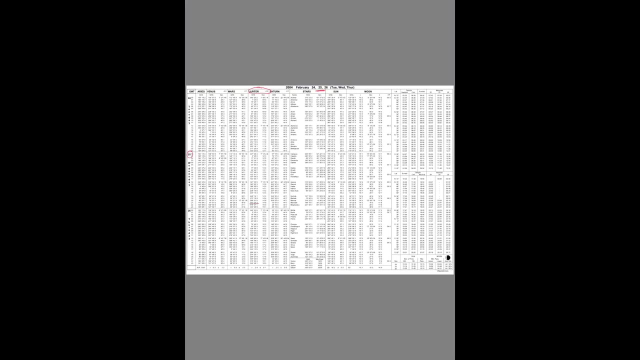 Alright, so let's find out where the LHA and the declination values are And where we can get the values from. So let's start by finding out the GHA value for 2100 hours of the sun. Alright, so I need to go into the nautical almanac. So if I go into the nautical almanac here for the 25th of February, 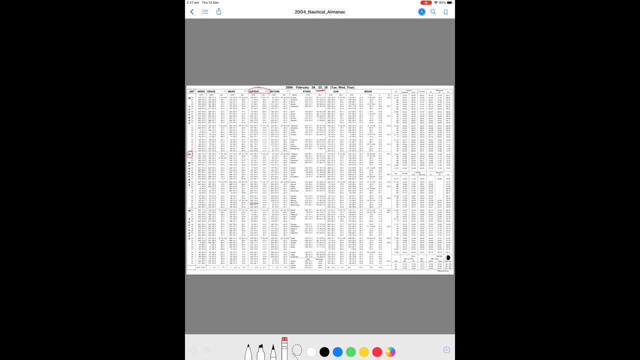 For the 25th of February. here you can see that. that's the date right on the top. What we have here is on the extreme left hand side. is the GMT time given to you, right? We need it for 25th of February. I need it for 2100 hours, right, I need it for 2100 hours. So I need to trace it all the way to the sun. The sun is here somewhere right? 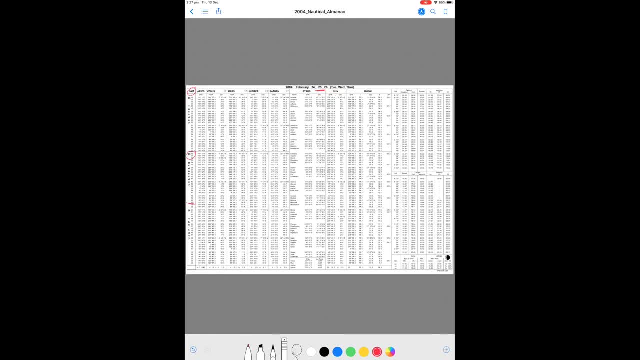 And you can see. I just circled it, but hopefully you can see that the GHA and the declination values are given here. right, You can see that this is the GHA and this is the GMT. This is the declination. So if I go down for 2100 hours, I need to zoom in here for you guys. 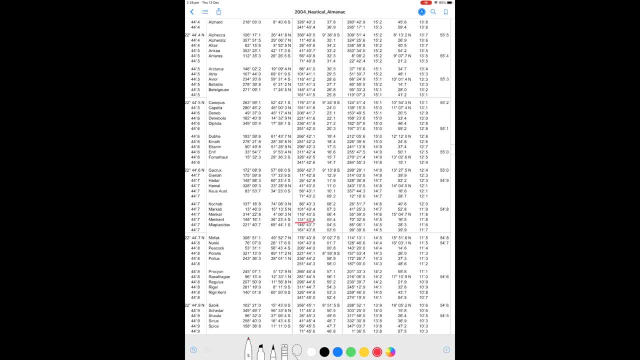 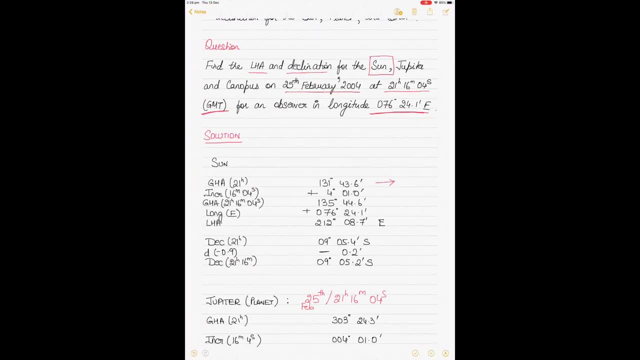 So the GHA value is 131 degrees 43.6 minutes. That's the value I need, So I'll go back and do my notes page. So 131 degrees 43.6 is what I have as a GHA value Now. I don't need GHA for 2100 hours. 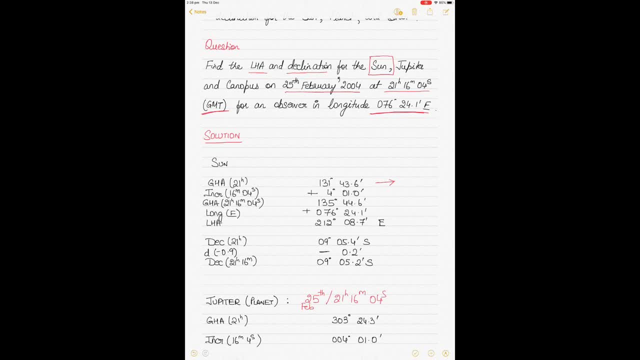 I need it for 2100 hours, 16 minutes and 4 seconds, And for that I need to apply a correction which is called the increment correction, And the increment correction can also be obtained from the nautical almanac. 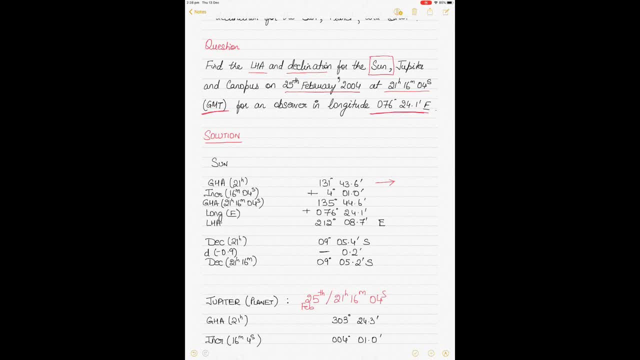 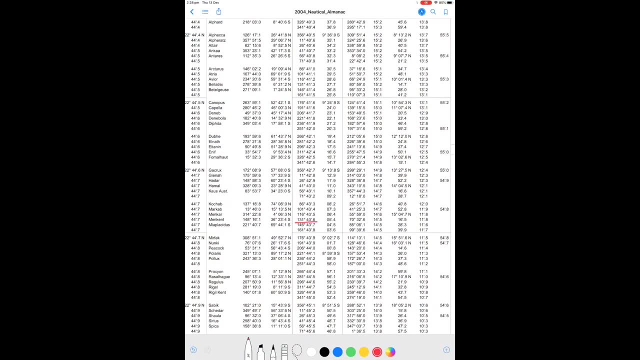 Increment pages are normally provided towards the end of the nautical almanac. They are known as increment pages. So if you go into those pages here for 16 minutes and 4 seconds, let's find out what's the increment. So, 16 minutes and 4 seconds, I'll go into the increments page here. 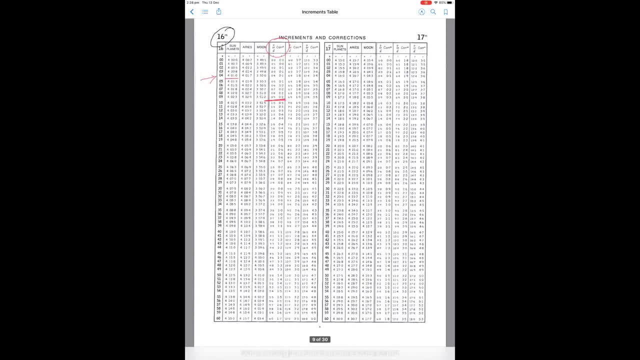 16 minutes and 4 seconds. So I need to erase the rest of this stuff so that you guys don't get confused. I've been trying to make this video a couple of times. That's why all those markings are there. So let's say 16 minutes and 4 seconds, So you've got 16 minutes here. You can see that that's 16 minutes, right. 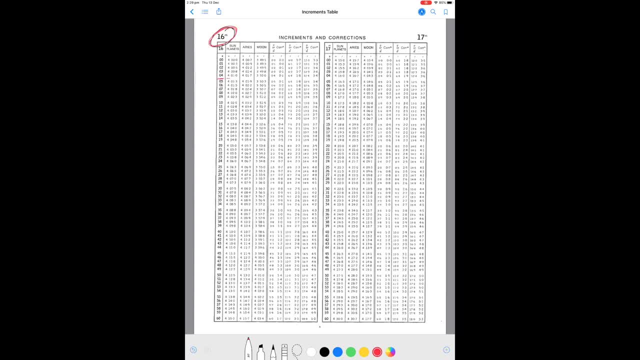 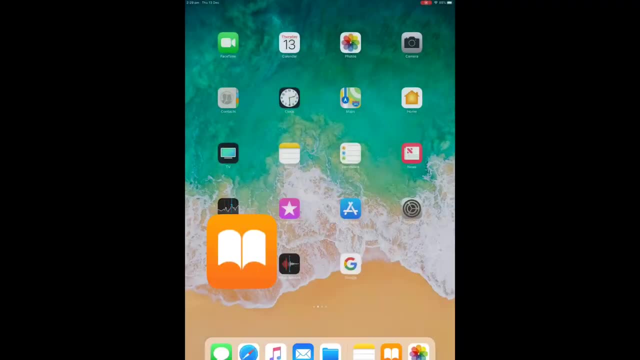 And for 4 seconds. seconds are given here. The increment value is 4 degrees 1 minute for the sun. So you get your increments for the sun and planets from the same column. So I'll go back out now and go back here. So 4 degrees and 1 minute is what I have here as the increment. 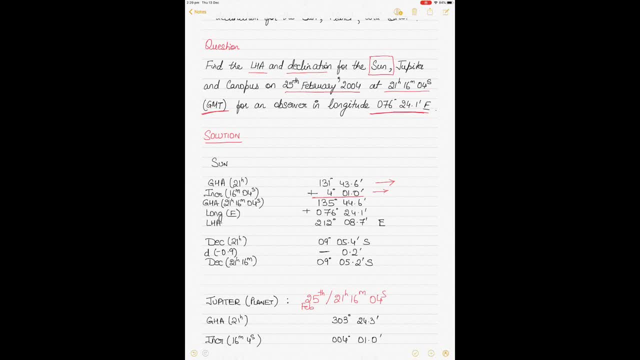 So I'll add the increment. Increments are always added. The word itself means addition, So we'll add it. And then we get the GHA corrected value for 2100 hours 16 minutes and 4 seconds. right With that we apply the longitude, So what we have is the east longitude. 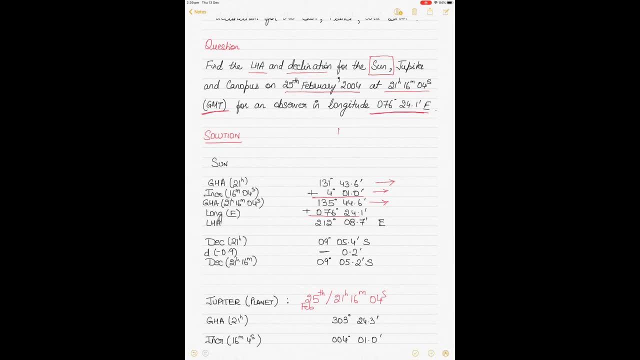 And the rule of thumb is that if longitude is east, right GHA is least. That means GHA will be less than the LHA. If the longitude is west, GHA is the best Right Now. towards the end, I will try to show you conceptually the relationship between longitude, GHA and LHA. 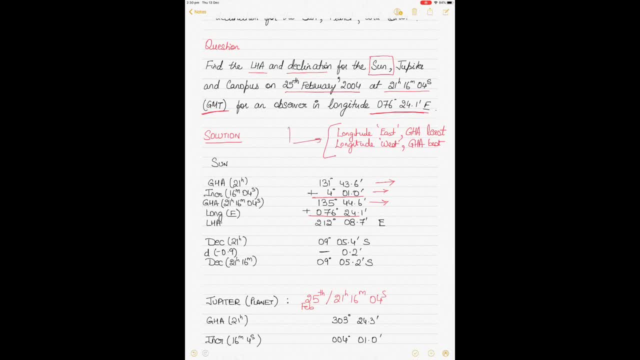 But for now, just remember this rule of thumb: to calculate your LHA from your GHA, applying the longitude. Okay, so, this is the rule of thumb you have to remember. That's a terrible one. So: longitude- east GHA- least. Longitude west GHA- best. 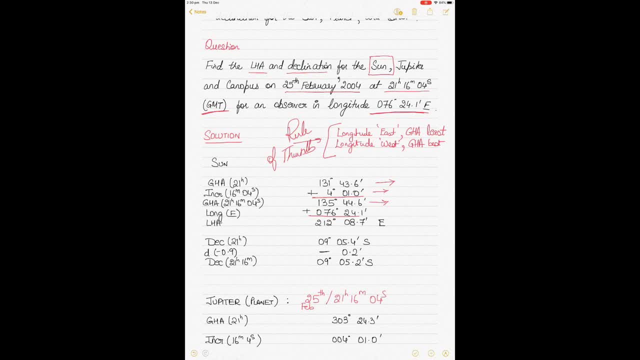 So if it's longitude east GHA is least, you need to add your longitude to the GHA to increase your LHA. In this case, that's what your LHA is Right Now. I have named it east Now in this context, naming the LHA is not important. 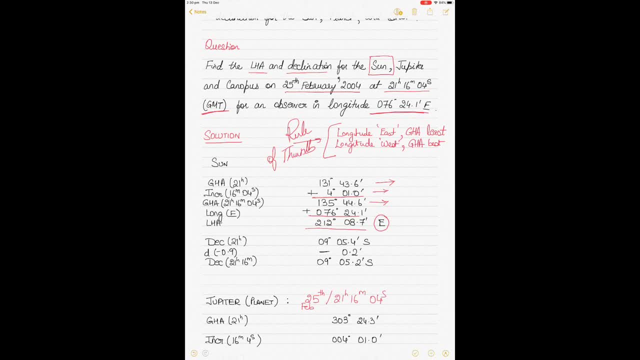 But what you will see in my other videos is when you calculate the compass error and you're trying to find the true bearing by calculating the components such as A, B and C, You will see that naming of the LHA becomes important there because you use it to name the other components of the calculation. 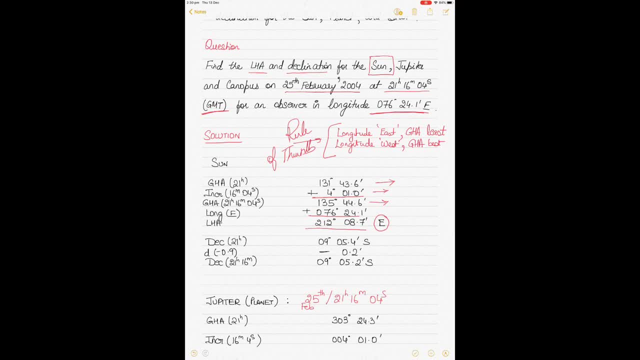 Right, Right, Right, Right, Right. So in this context here you don't have to worry about naming it, But I'll teach you how to name it, because there's another rule of thumb here. There's another rule of thumb. 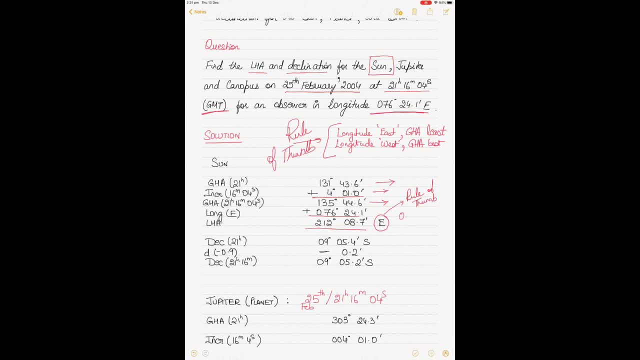 And the rule of thumb is that if the value of the LHA is between 0 and 180 degrees, then you name your LHA west. If it is greater than 180 and to 360, you name your LHA east. Alright, so later on, when I show you conceptually the relationship between longitude and GHA and LHA, you will get a better idea of why it is so. 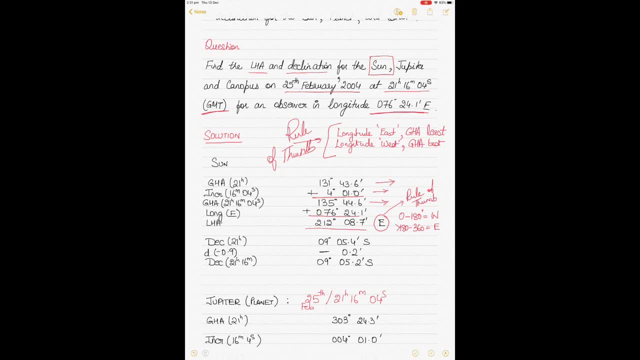 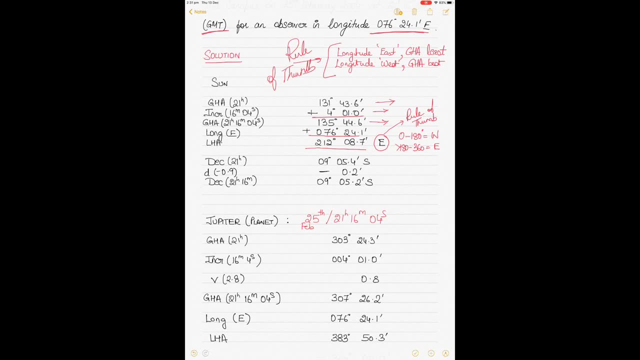 Alright, for now, Just remember this rule of thumb. Alright, So I have this rule of thumb written on the screen here so that you can remember it. Write it down. So these are the two rule of thumbs that we use here. Alright, so you got your LHA now. 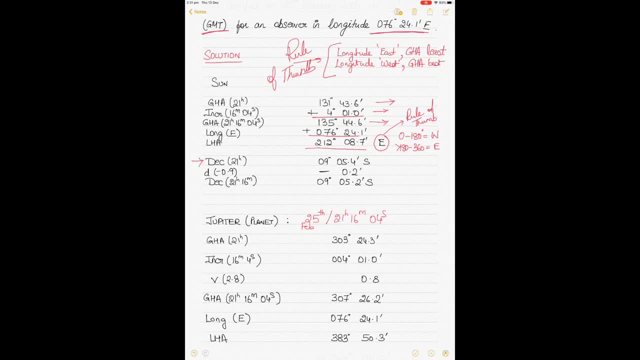 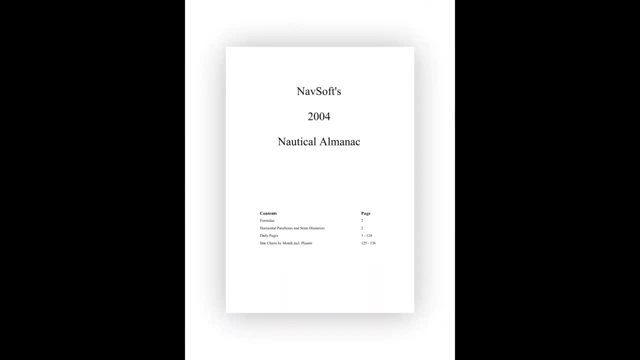 We need to go back to the nautical almanac and find the declination value for 2100 hours for the sun. Alright, So once we go back, we go back into the nautical almanac, page 2100 hours. 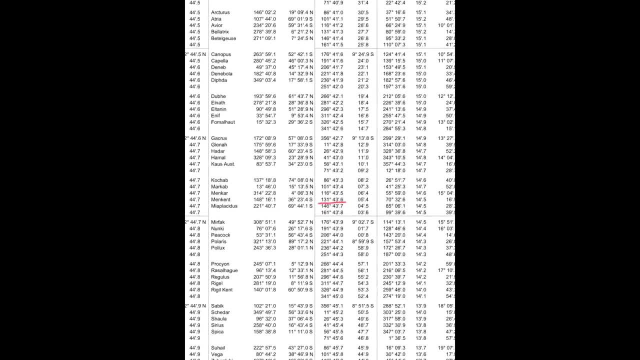 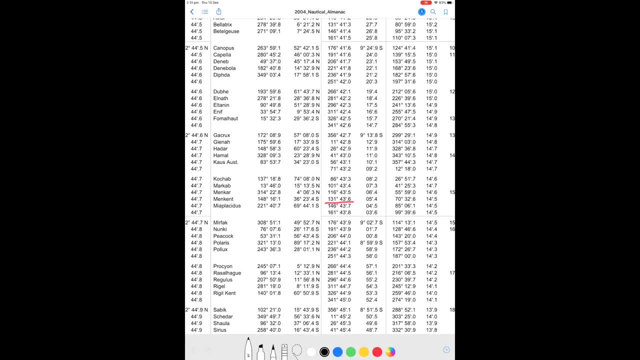 So right next to the GHA is your declination value. So if I zoom in here, you can see that the declination value is 9 degrees, 5.. 9 degrees, 5.4 minutes south. Right, You see 5.4 here, but you can see the 9 degrees here. 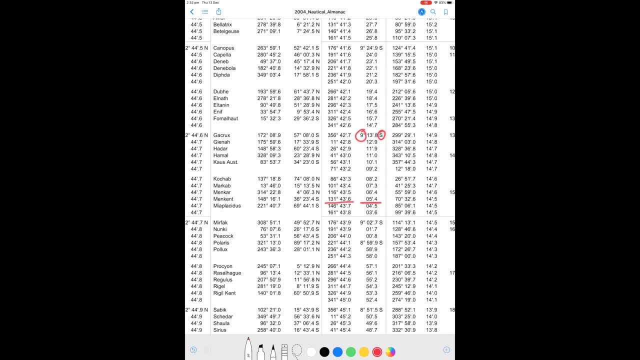 You can see the south here, Just in case you were wondering where I got my 9 degrees and 5.4 south from. So that's your declination value. But while you are here on this page, note down a couple of things. 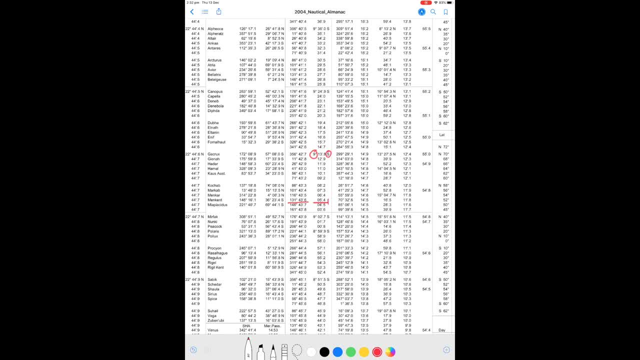 The first thing that you note down is that as you go from 2100 hours to 2200 hours, you can see that declination is decreasing. This is important because now you got to apply a correction to this declination. So you need to apply a correction to this declination value to get the declination for 2100 hours 16 minutes and 4 seconds. 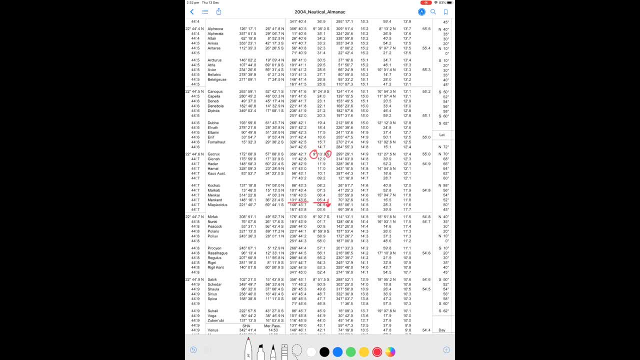 So if the declination is decreasing to the next hour, the correction that you obtain needs to be subtracted from this value. So this is the declination value: 9 degrees 5.4 is for 2100 hours, Right. 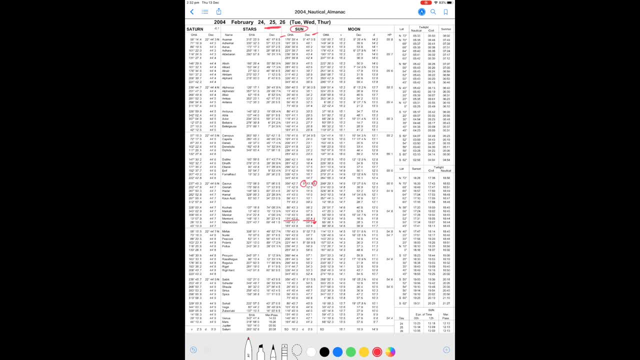 So you need to apply a correction. Now what is a correction? Correction is called de-correction, but this is not the value you apply. You use it and go into the increments page to find the de-correction value. So this is the de-correction value to go into the increments. 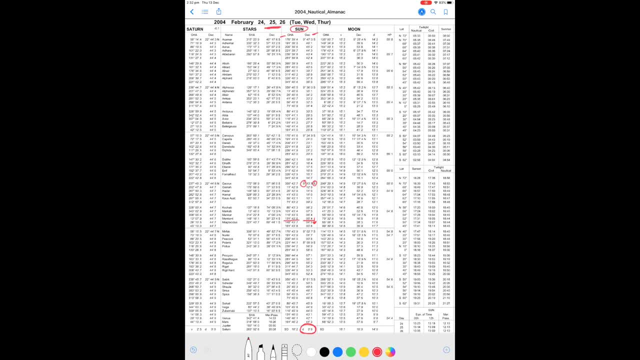 So the de-correction value here is 0.9.. So these are a couple of things that you note down. So, firstly, we note down the value of the declination here, which is 9 degrees 5.4 minutes south. 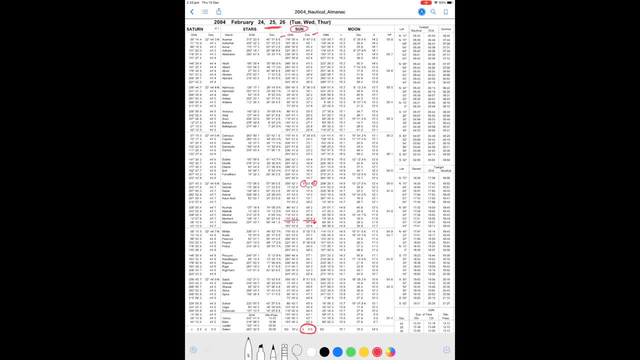 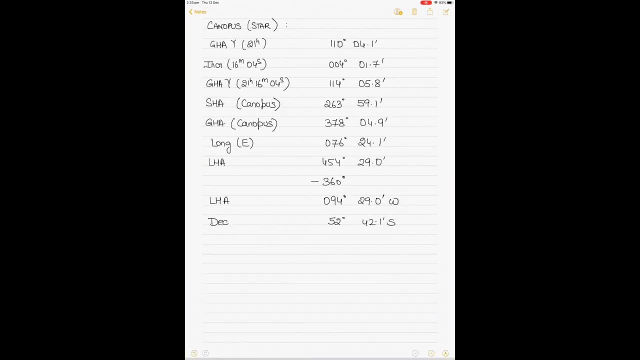 You note down that the declination is decreasing to the next hour and you note down the de-value. So with that we go back into the notes page and this is what I have here. Declination is 9 degrees, 5.4 minutes. apologies, such a big shift. here you go. 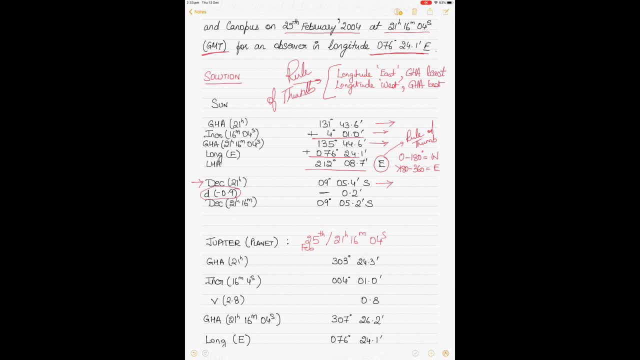 The de-value that I got from the bottom of the nautical almanac was 0.9.. Now it's a negative sign because, like I said, it was reducing, so it needs to be subtracted. Now, where did I get my 0.2 from? 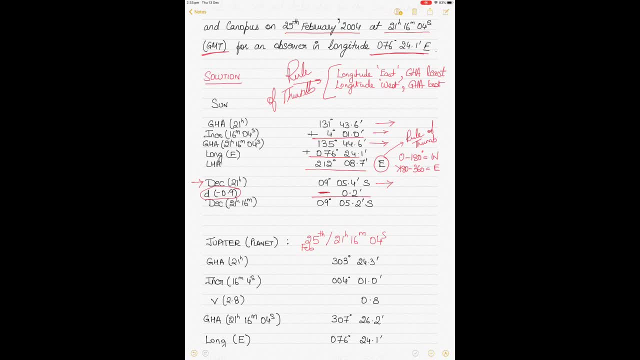 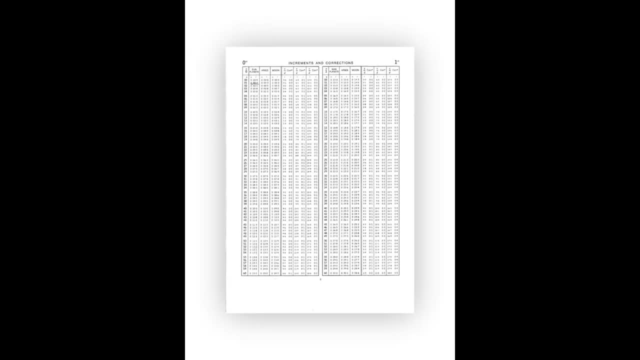 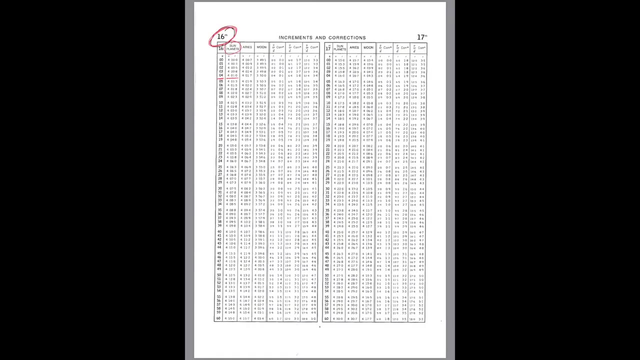 Now I used this 0.9 to go into the increments page for 16 minutes, alright, And this is where I go back. So I need to go back here and I go back to the increments page, alright, Alright, takes a few goes. 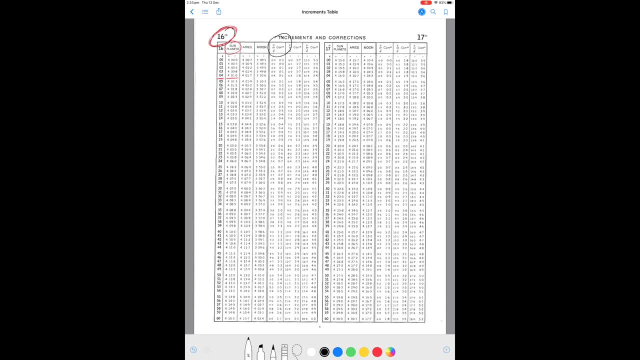 Now, if you see the column here, it says V or D correction. right Now. this is where you take your de-value. you go down the right hand side column and you see the de-value is 0.9 here, the one that you got from the bottom of the almanac. 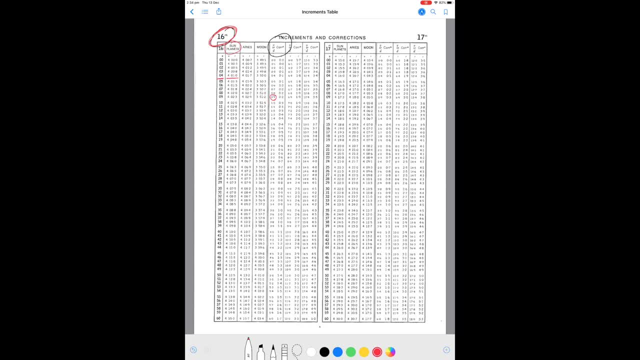 page on the 25th of February. Next to it is the de-correction value, and that is 0.2.. So you use this value, 0.2, and apply it to our declination. Alright, so you go back and see. this is what I have done. 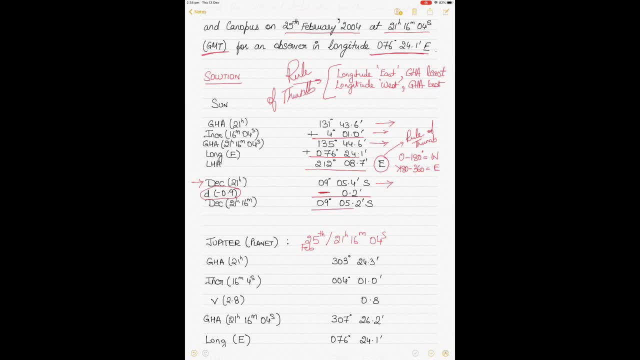 I have applied 0.2. And that's how you get your declination value for the sun, And this is for 2100 hours, 16 minutes and 4 seconds. Alright, so the principles pretty much remain the same for the planet and the stars. 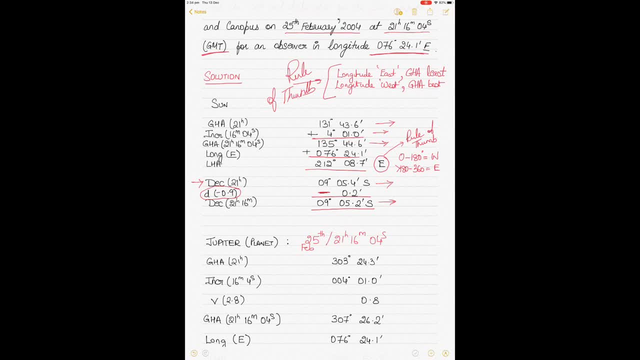 I will take you through them as well, but the principle remains the same, except for a couple of corrections here and there. Alright, so remember these rule of thumb, remember the principle that we used to apply for declination correction and obtaining the LHA from the longitude and the GHA, and with that we will. 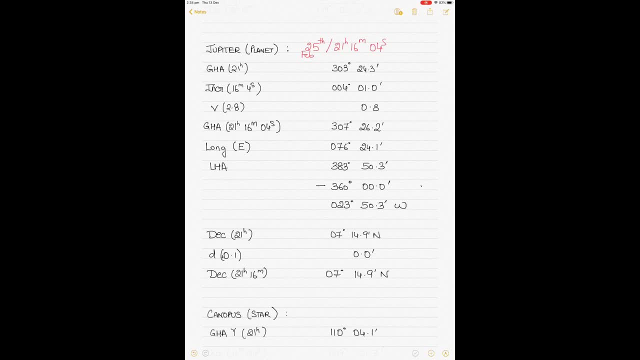 go into the next example For the planets. now the planet example. the date and the time is same. I need to go back to the 25th February nautical almanac page to get the GHA value alright for 2100 hours. 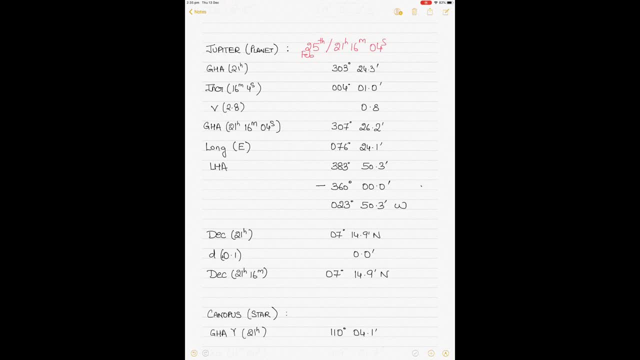 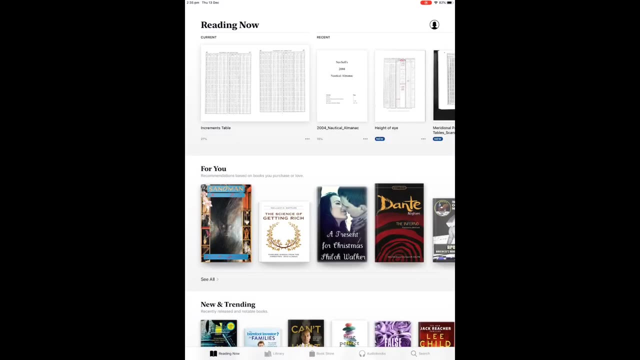 So the same, it's the same principle, like we did for the sun, except that now we go into a separate column. So this is planet and this is Jupiter. So if I go back out from here and I go into the nautical almanac page for 25th of February, 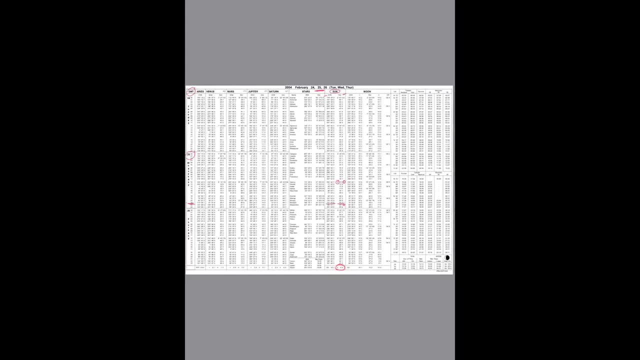 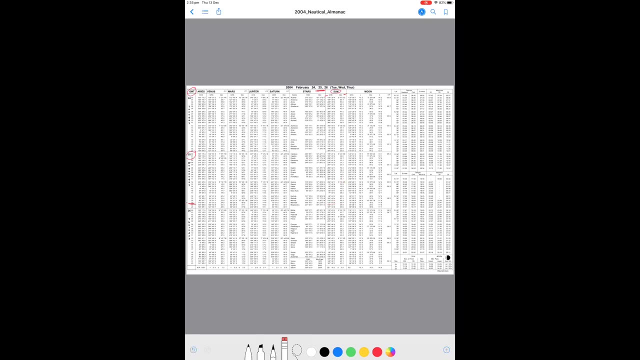 I need to erase the rest of the stuff. Hmm, Alright, There you go. Thanks for bearing with me. I will erase the rest of the stuff here so that you guys don't get lost here what I'm doing here, So you can see that the planet's column is given for Jupiter, of course, is given here. 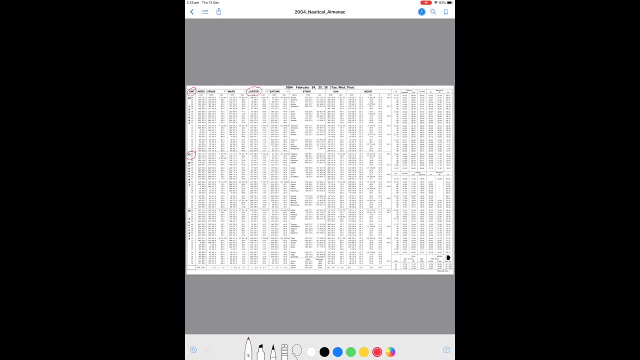 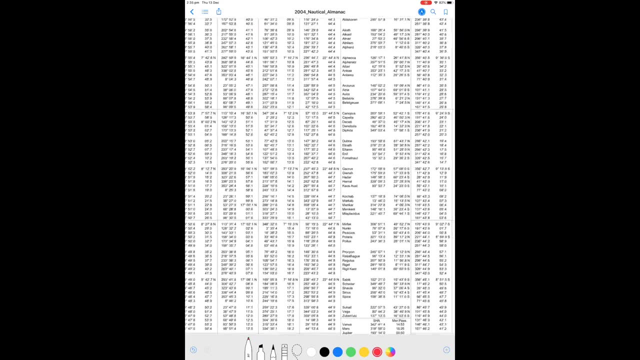 right, The principle remains the same. We go down the 25th February date and this is the 2100 hours. and if you see, if you really focus on the 2100 hours, and if I zoom into the value of the Jupiter here, your declination. 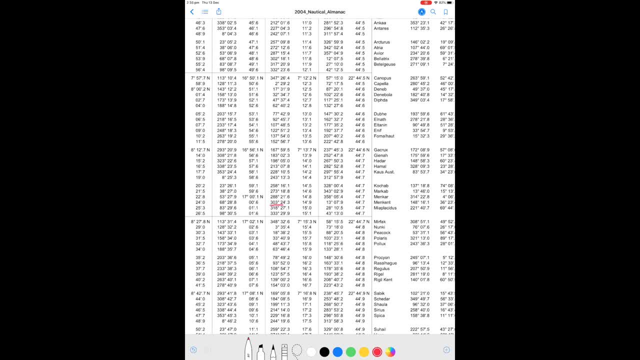 value. sorry, your GHA value is 30324.3,. right, While you are it, or while you are at it, or while you are on this page, note down the declination value as well, because now you know the rest of the stuff. 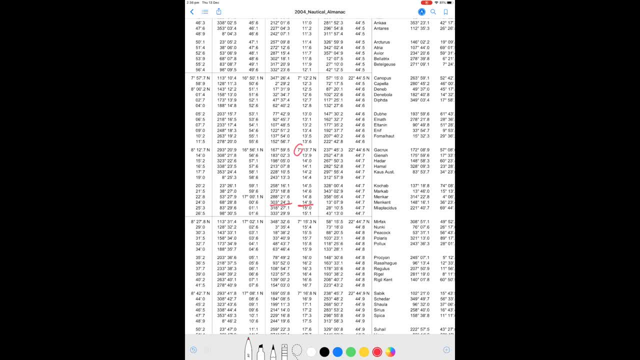 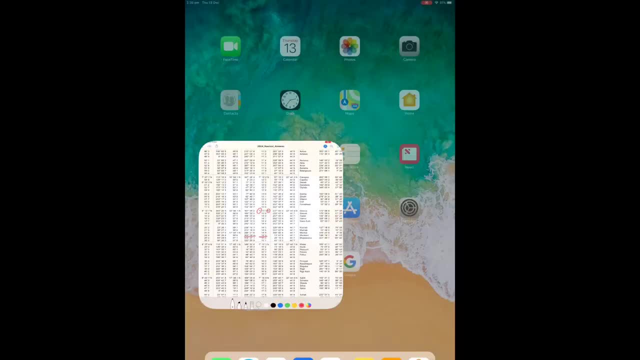 Just note down the declination value as 7 degrees 14.9 minutes north, Alright, So 30324.3 and 7 degrees 14.9.. 30324.3 and 7 degrees 14.9.. So you have 30324.3 here. 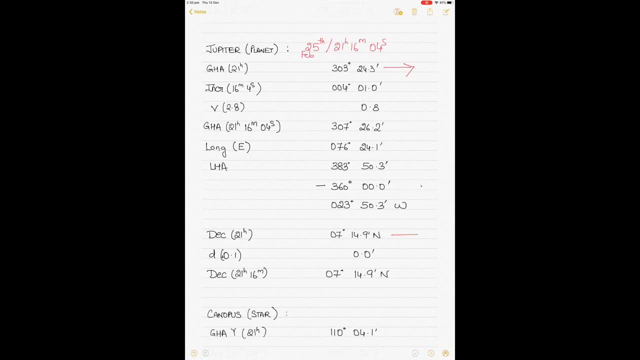 I have noted down the declination value well before 7 degrees, 14.9.. Alright, We go back to the increments page. now I am doing two things at a time, alright, So because you know the principles already, so I am just trying to save some time here. 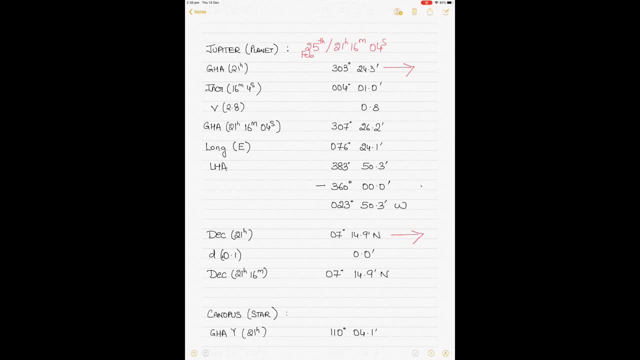 So, but I think I might confuse you here. So let me handle the GHA first, or the LHA first, and then I will go back to the declination. right? So we have got the GHA value now, Okay, And we need the increment for 16 minutes and 4 seconds for the planet. 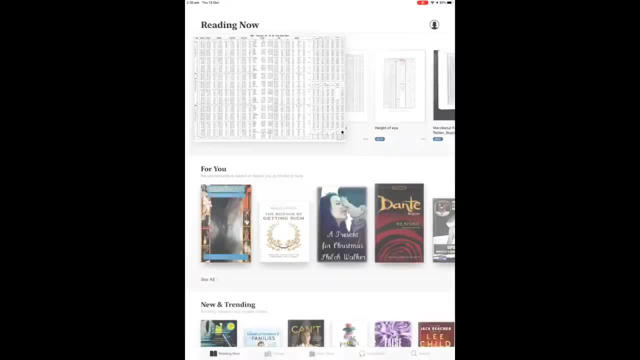 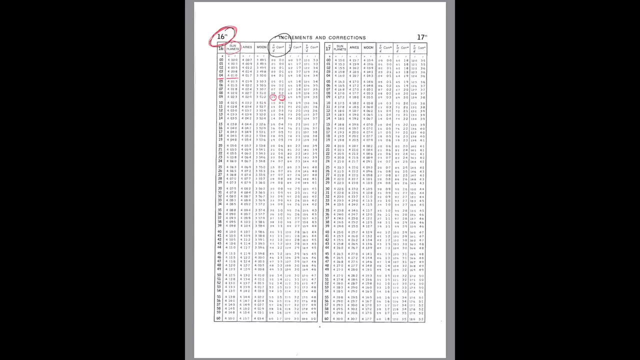 So you know what to do now. Just go back into the increments page. I need to move out of this page here. Go back into the increments page for 16 minutes and 4 seconds. It's the same as planets. You can see that the column remains the same. 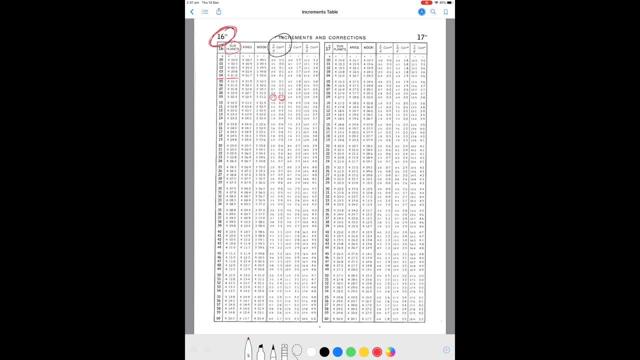 And that's why it's still 16 minutes and 4 seconds. The sun and planet's column is the same. The value is the same: 0404 seconds. It's 0401.. Alright, So I can go back out of here. 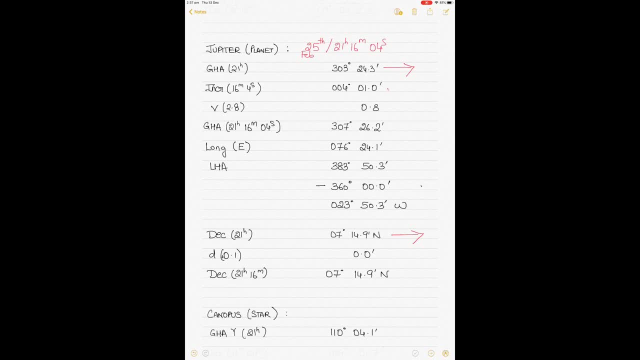 Go back here And 044 degrees and 1 minute is what I have here, Right. So now I will add this value because it's an increment value. I told you before increments are added: An additional correction for the planets is a V correction value. 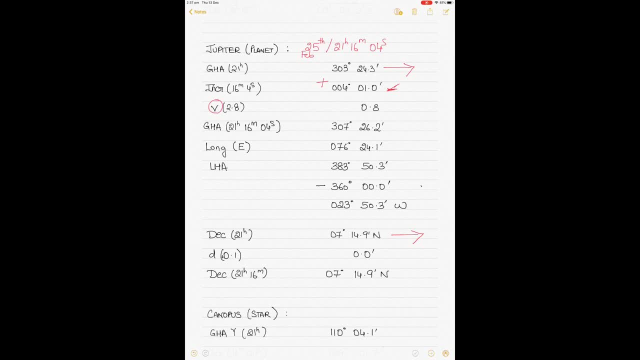 Now, what do we get? Now, where do we get this V correction from? Alright, To get this V correction, we need to go back to the nautical almanac for the date of 25th of February, And I can show you from where I get that. 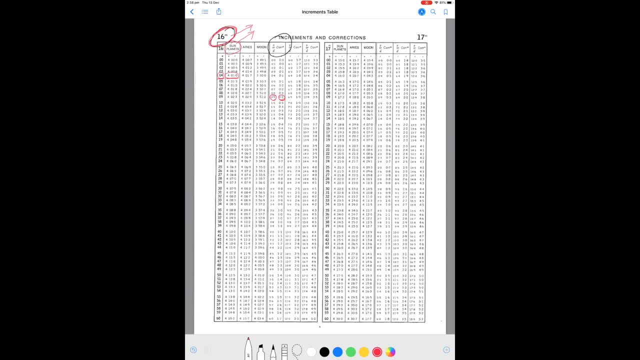 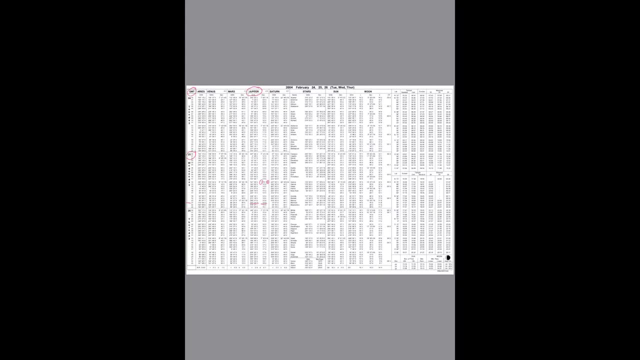 Alright, So what we do is we go back here. We need to move out of this page here and go back to the nautical almanac here. Sorry about this to and fro, This is the best way I can show it to you. 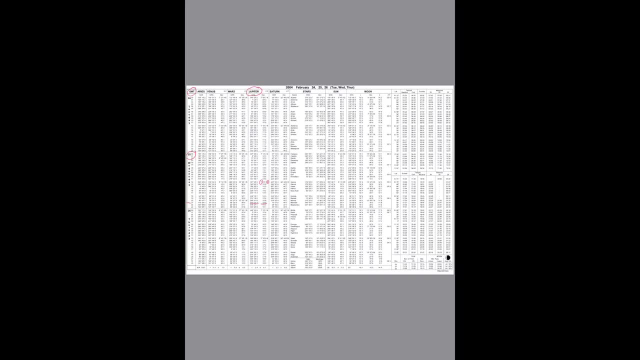 So what you see here is that for the planet of Jupiter, if I can show you here, is that there is something called V correction at the bottom of the page of the GHA Right. So if you see here, I will highlight it to you. 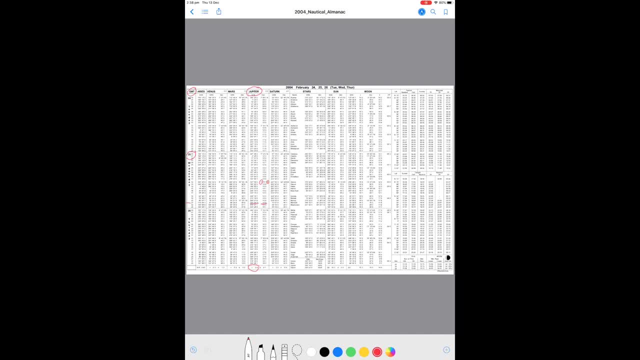 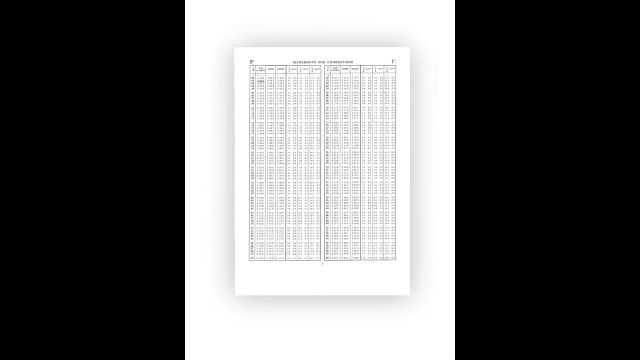 At the right of the bottom of the page is your V correction as 2.8 and also your D correction as 0.1.. Alright, So with that V correction of 2.8, you need to now go into the increments page and for 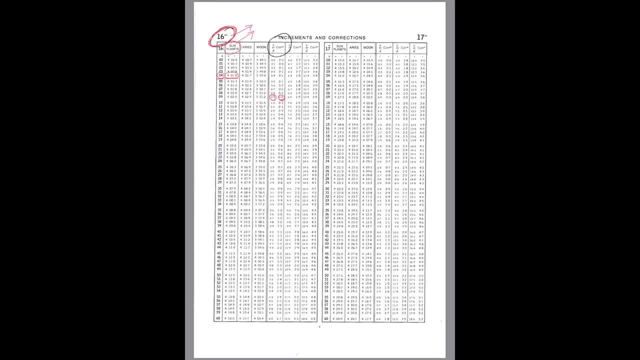 16 minutes. So for a V correction value. So you can see the V and the D's are given together and this is your V and D's right, Your V and D correction. So this time you need to find it for 2.8.. 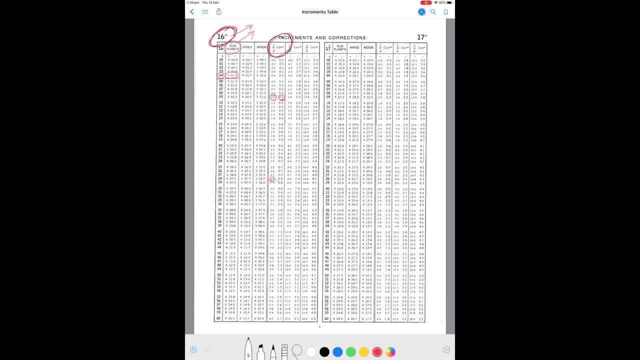 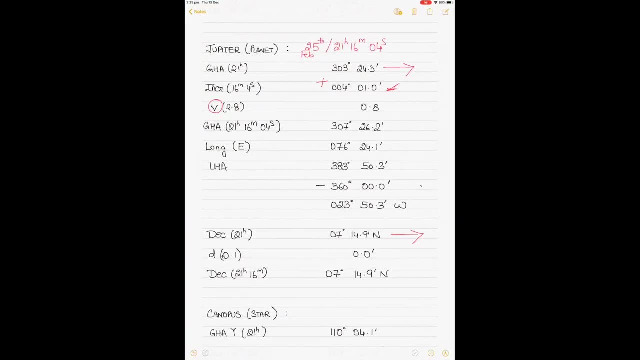 You can see 2.8 is here. This is your V value: 0.8.. This is the correction that you apply to your GHA when it comes to planets. This is what I have done here. I have got this correction here. 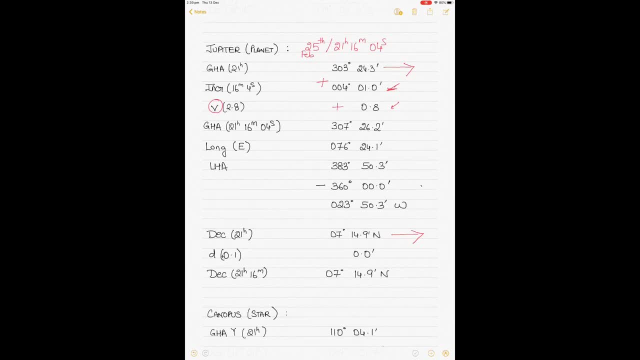 This is added as well, This will be 26.1.. Alright, So let me erase it and write it properly so that you guys don't get confused: 26.1.. So this is V2 as well, Right? So if I add it, you will get 26.1.. 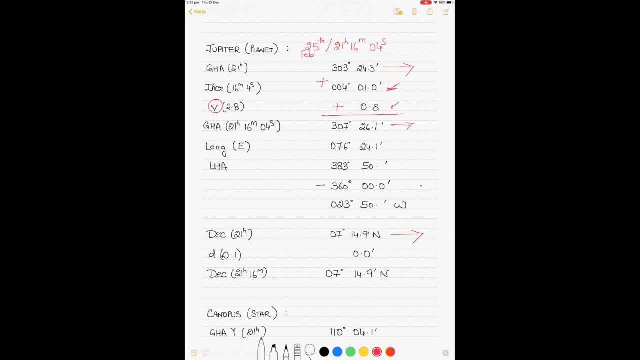 307 degrees. 26.1 is the corrected GHA. You apply your longitude with the same rule of thumb that I taught you before. Longitude East GHA is least, So you will add your longitude to the GHA. In this case the LHA becomes greater than 360, and that cannot be the case. 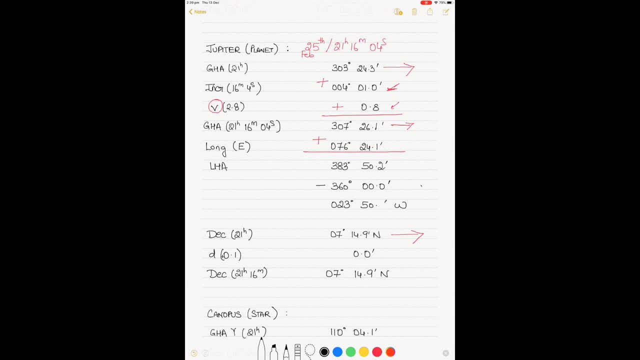 So if LHA is greater than 360, you need to subtract it from 360.. Alright, Because LHA cannot be greater than 360.. So if it is greater than 360, you will need to subtract it from 360, as I have done before. 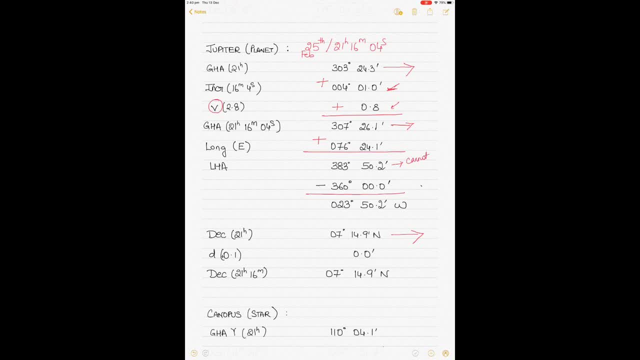 So LHA cannot be greater than 360 degrees. And that's how you get your LHA value. I have named it West again, as per the rule of thumb, If it is between 0 to 180,. if it is between 0 to 180, then of course you name it West. 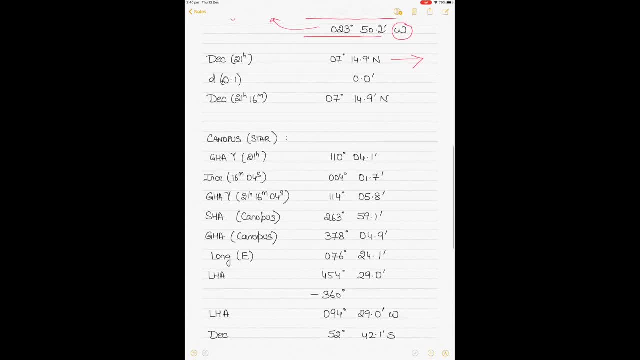 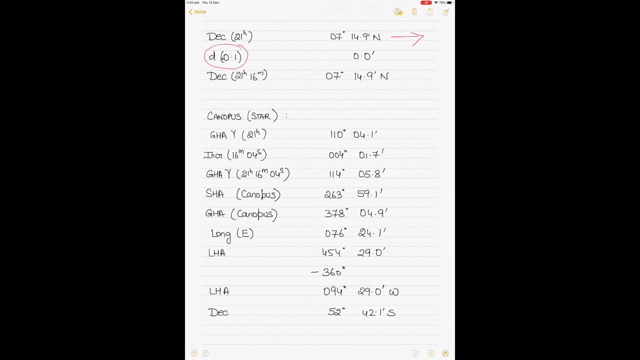 Alright, Now I will come back to the declination value. You all know where we got the declination from: It was next to the GHA. You know where I got my D value from: It was next to the V correction value at the bottom of the page. 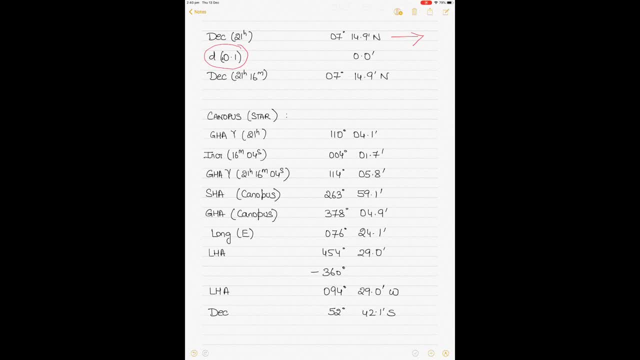 In this case, here we go back. We go back to the nautical almanac for 16 minutes to get a D correction value. This is a D value and we need to get a D correction value for 0.1 for 16 minutes. 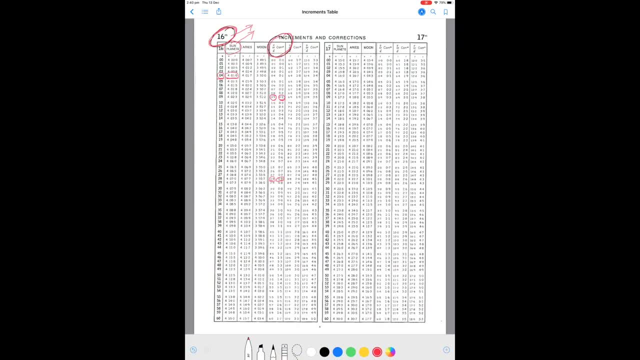 So if I go back here for 0.1, you can see that the value is 0. Right, So there is lots happening here. So you guys are probably getting confused with all these values that are being highlighted. So I will take off all these values. 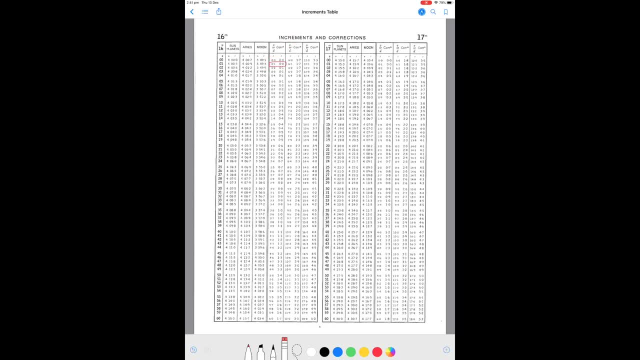 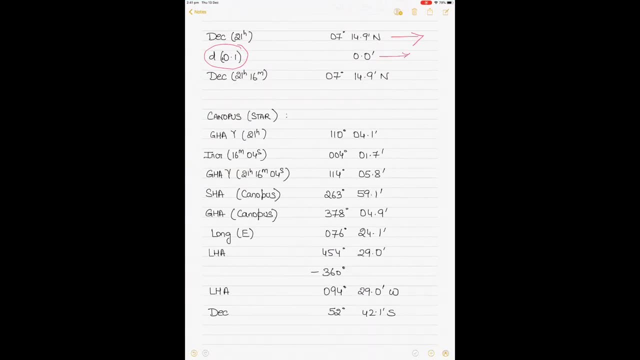 Alright, Just keep this here So you can see: for 0.1, it is 0. So I will go back here and I will apply the 0 here. So it is insignificant now, In this case it doesn't matter whether it is plus or minus. 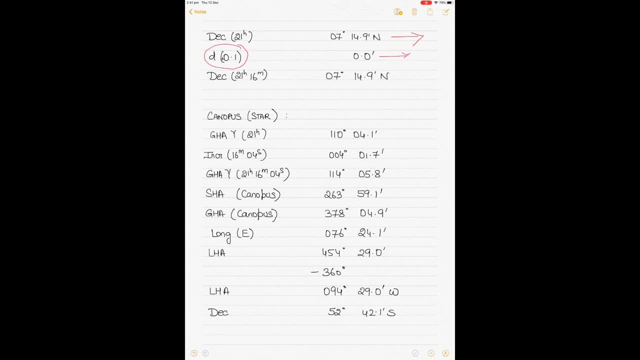 But if it was decreasing, you would add it. If the declination was increasing to the next hour, you would add it, And if it was decreasing to the next hour, you subtract it. You remember the concept Right. So in this case, of course, it is 0. 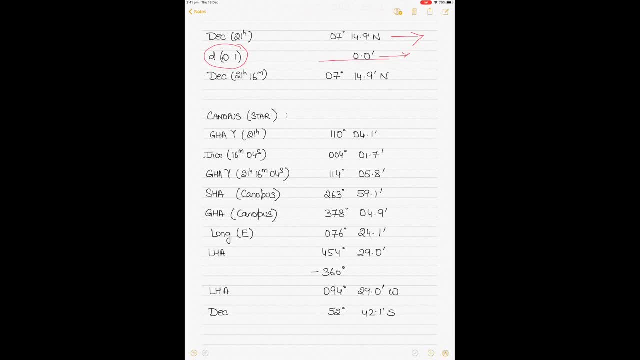 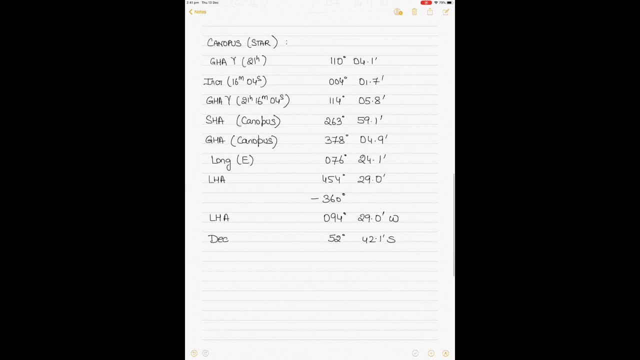 It doesn't matter, So it is insignificant. So the declination that we get for the planet is 7 degrees 14.9 minutes north. This is a planet Right Now. similar concepts again. This time there is no V correction. 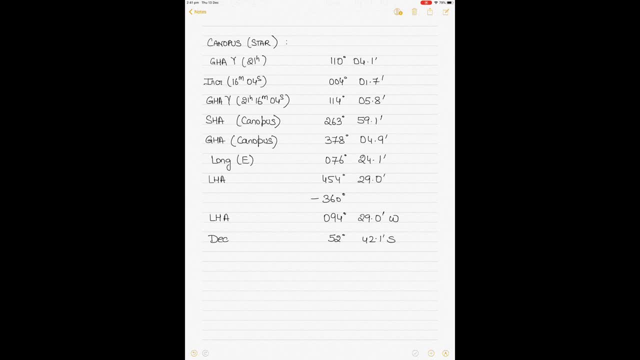 But there will be an additional correction called the SHA, And we will see how we get that one too. Alright, So the star in this case is Canopus. This is an example of a star Example, And we need to find the LHA again. 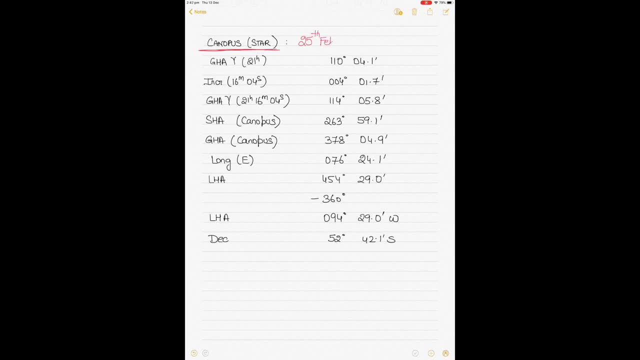 For 25th of February is the date And if I write down the time, the time is 1621 hours. I am sorry, Not 16 hours, but 2100 hours And 16 minutes and 4 seconds. And you need to find the LHA value of the star and the declination value of the star. 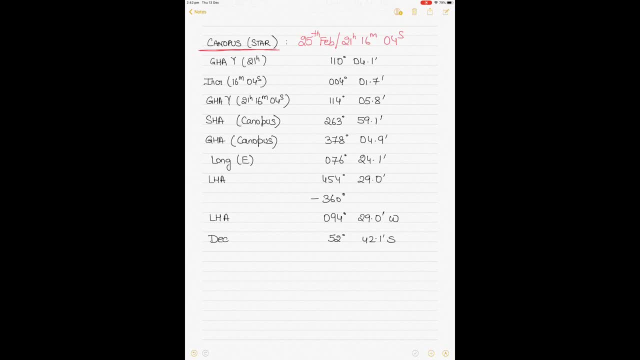 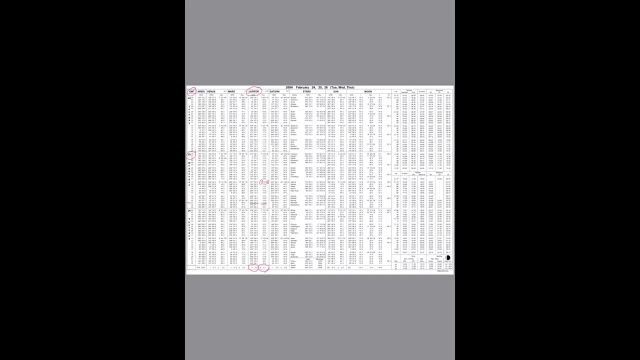 Right, So it is for Canopus. So let's go back into the nautical almanac And I will go back. So I need to get rid of a little bit of all these markings, Otherwise you guys are probably getting confused with all this that is happening here. 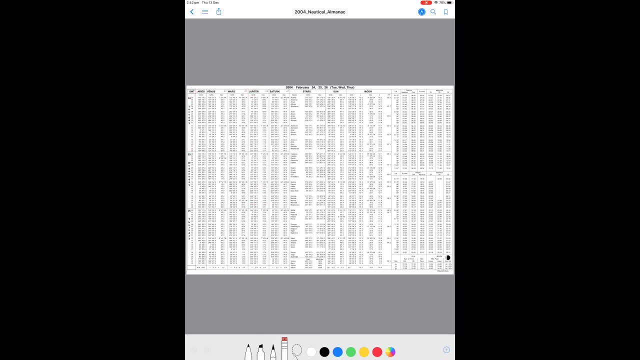 So I will get rid of all these markings here Right And I will start fresh for the star. So the star. as you can see, There is nothing called star, But what you have here in the extreme left hand column next to the GMT column, is something. 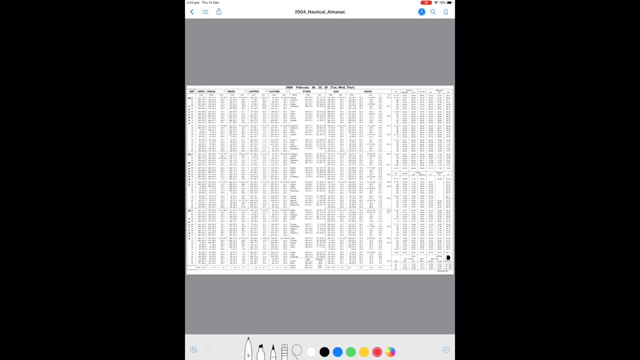 called the Aries. This is what we use for the star, So this is the column that we use. So we have our 25th of February here, We have our 2100 hours here. For 2100 hours, your GHA is 110 degrees, 4.1 minute. 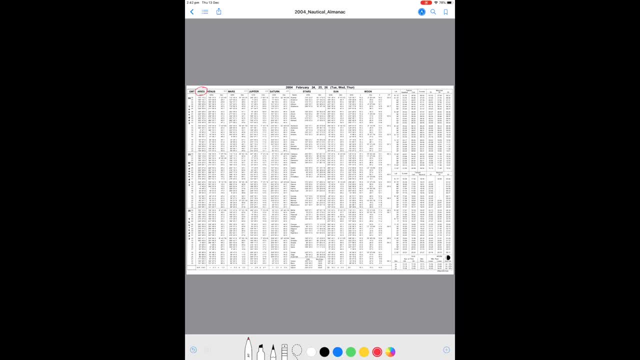 That's the one that we take Right, We go back And we go back here 113.. So we have our GHA is 110 degrees, 4.1 minute. That's the one that we take Right, We go back. 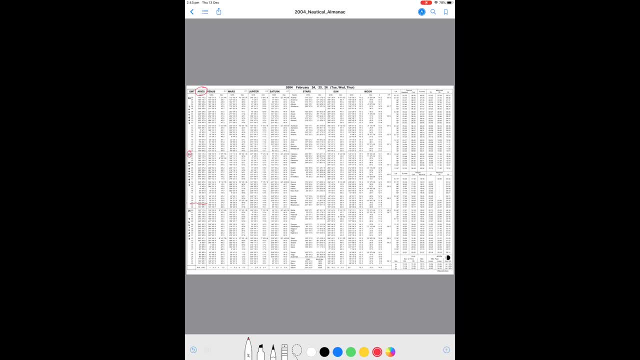 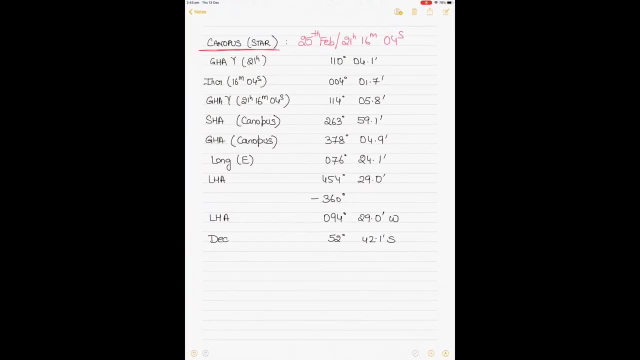 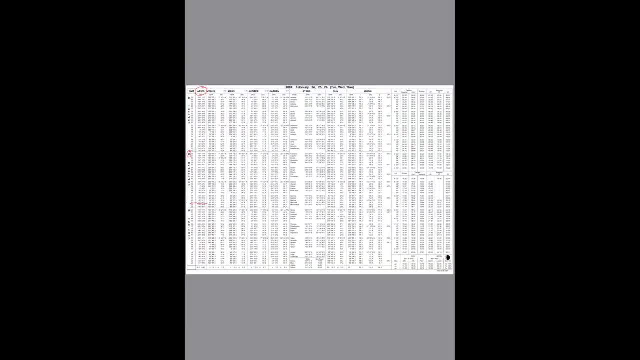 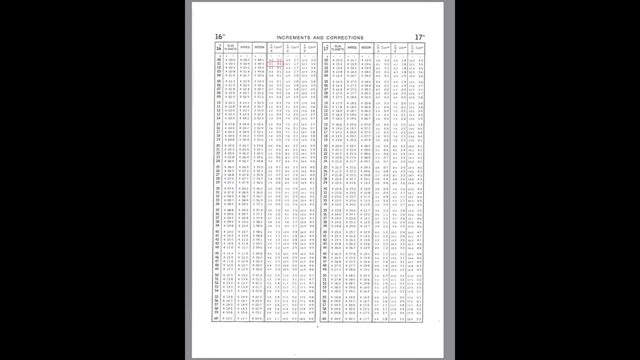 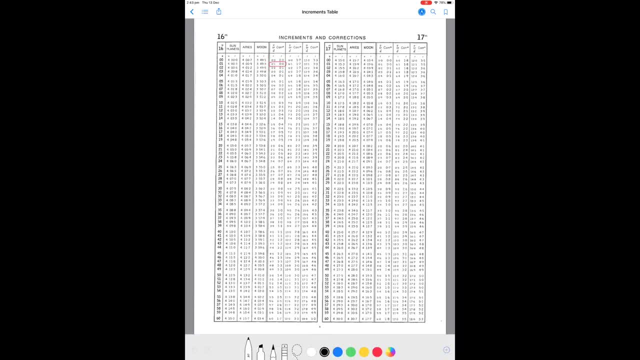 And we go back into the increments page for 16 minutes and 4 seconds and I need to move out of this page. Go back into the increments page for 16 minutes and 4 seconds, If I can bear with me, Okay, Thank you. 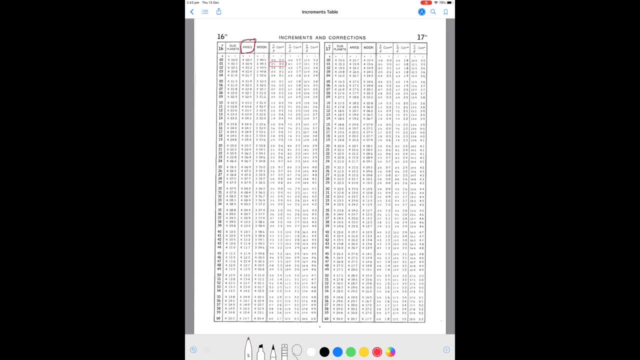 So 16 minutes and 4 seconds for aries, you find out the increment value, which is 4 degrees 1.7 minutes. that's the value you take, all right, so let me get rid of the rest of it. 4 degrees 1.7 and i move out, go back here and 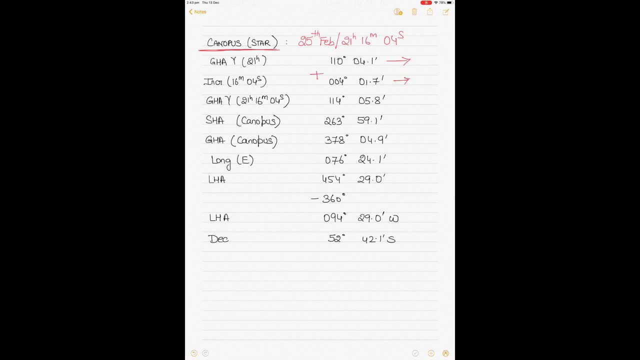 that's what i have here is the increment. increments are always added, so you will add to it and that's the gha corrected- gha aries corrected. right now, here you have to apply an additional correction before you apply the longitude straight away, and that's called the sha sha star. 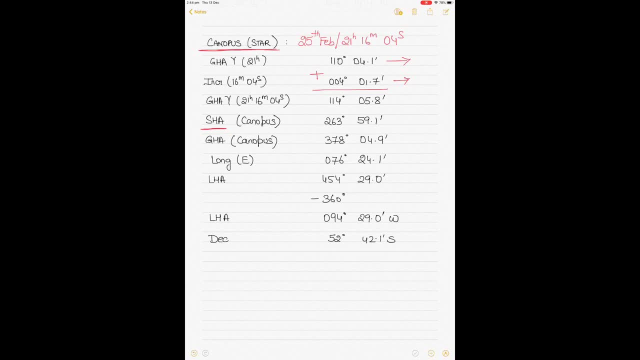 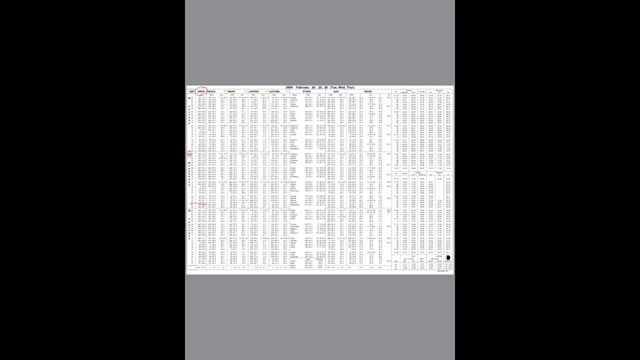 sha stands for sidereal hour angle. all right, so what we do is we will apply the sha of the particular star canopus, and to do that we go back into the nautical almanac for the date of 25th of february, we move out of the increments page, we go back to the nautical almanac page and you can see. 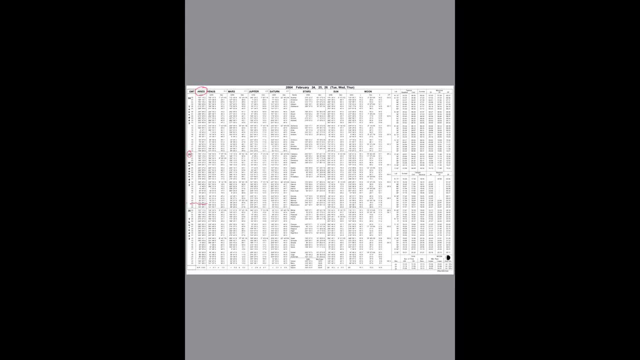 that somewhere here- let me show you where you all right, somewhere here is the stars right- switch us back to black all the time. so somewhere here is the star and this is the sh and this is the declination. so let me erase it so that you can. 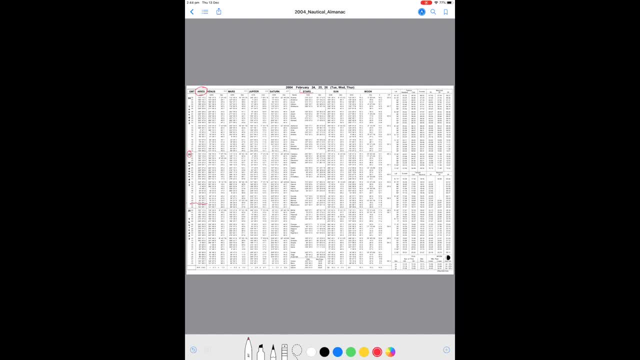 see it again. so this is the star right in the center here, right, you can see it. and then you have got your sha and your declination values here for each and every star. this is in alphabetical order. now what i need it for is a star called canopus, and this is the star called canopus. 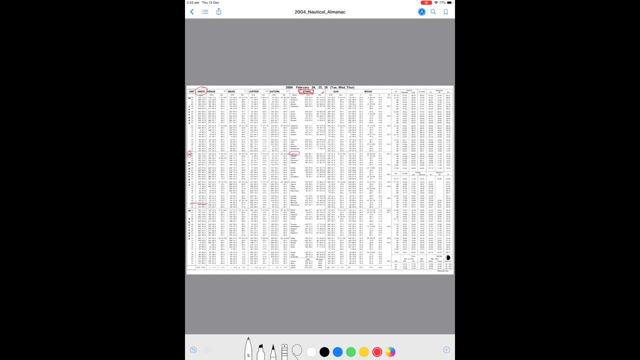 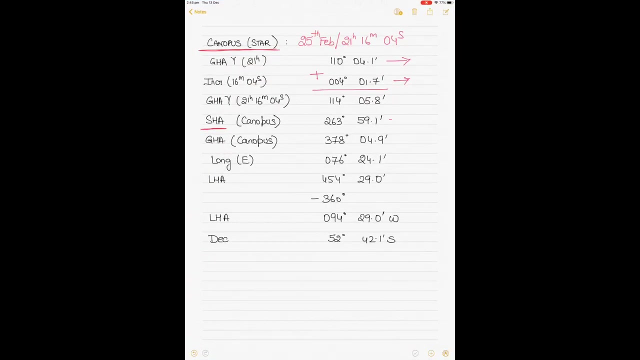 and canopus is here and i have got my sha value and my declination value right next to each other so i can note down both of them. the sha value is 263, 59.1 and the declination value is 52 degrees, 42.1 minutes south right. so i go back write it down. i've got my sha value here and i've got my. 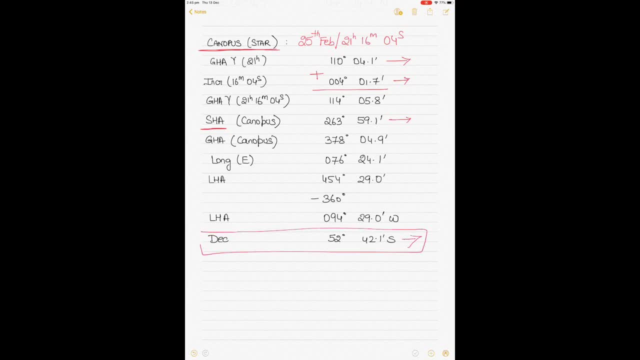 declination here. now i can finish off with the declination, because we're going to have to do this. when it comes to star, there are no de-corrections required. star is too far to have any de-correction values. the rate of change is very slow, so the declination is very slowly changing. all right. 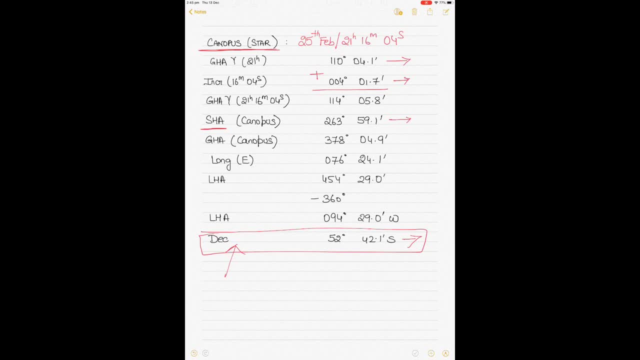 so that's why we just straight off, note off, and we can finish off with the definition regarding the sha. sha is always added to the gh, irrespective, so you always add the sha, never subtracted. now, once you add it, you can see that the value comes out to be more than 360. 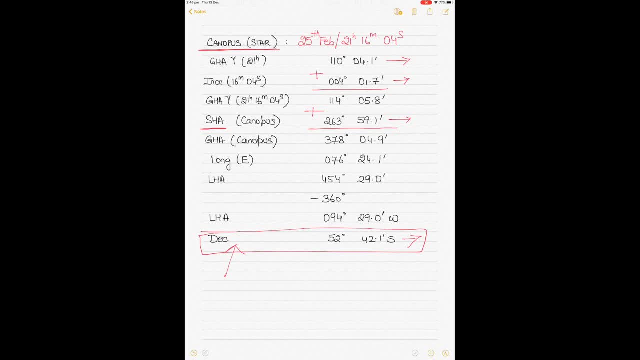 all right, so you can straight off subtract 360 from here, or you can wait and see what to do with the longitude and then subtract 360 later. now, in this case, because your longitude is east and you know the rule of thumb, longitude east is gh at least, and since you will be adding the longitude, your 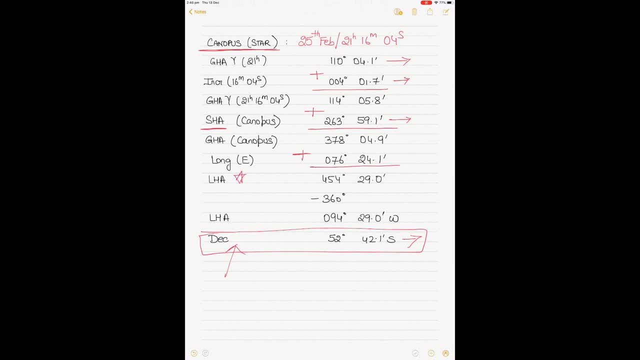 total lh star value. this is how we write. lh star comes out to be 454 degrees 29 minutes. now, since this cannot be more than 360, cannot be more than 360 degrees, why you subtract 360 from here? you could have done this. you could have done this subtraction at this. 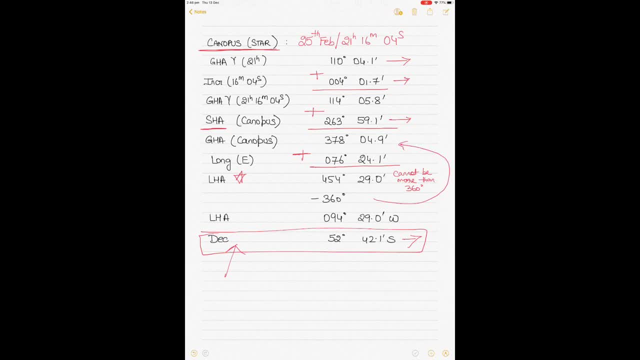 stage as well. it would have been the same thing, but we waited and we added the longitude because it was to be added, and then we subtracted 360 and you would get the same result and you get the lha. so that's how it is. pretty much it's the same principles, except that with star you have an. 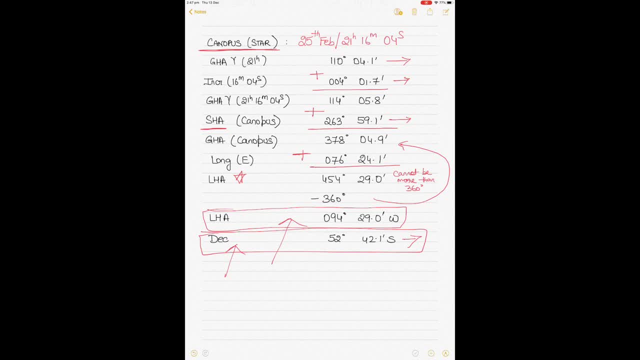 additional correction called sha. with planets, you have an additional correction called the v correction, which is applied to the gha and with sun. of course, you saw that the corrections are the basic corrections there. so go through these videos, go through these different examples again and see what are the 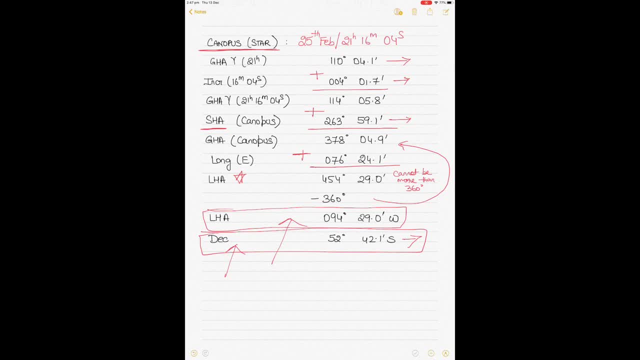 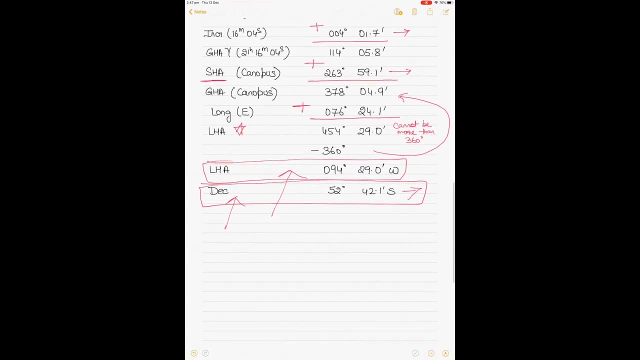 corrections, and how do they differ from one another? you need to go a bit back and forth with the nautical almanac, as i have, but before i finish off this video, let me show you the relationship between longitude gh and lh, as i promised before, and for that i need to make a 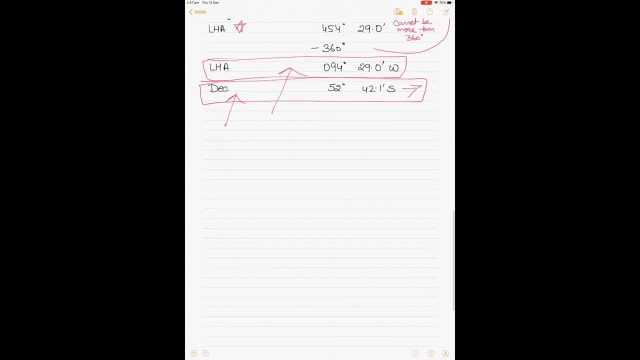 circle, and my apologies if it looks really ugly, but i'll try my best here. all right, so if you make a circle here and imagine this to be the spherical part of the celestial sphere of infinite radius, right now i'll start: the gha. the gha is the. 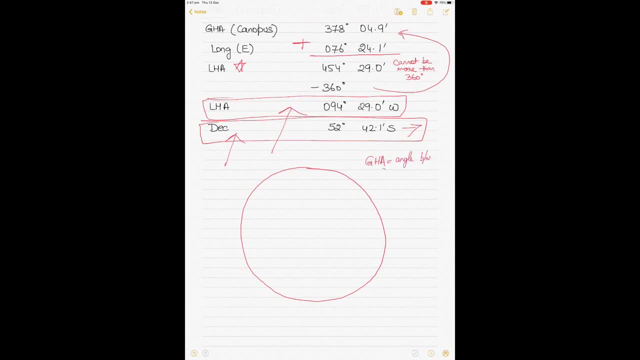 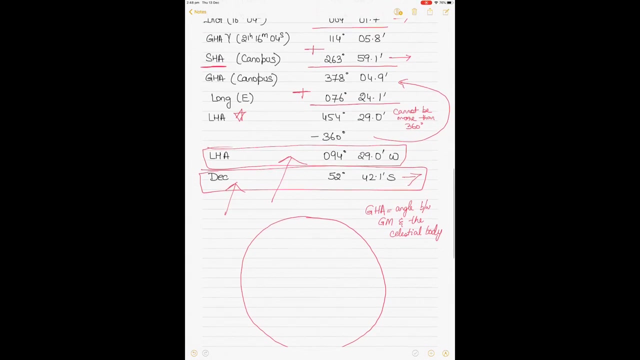 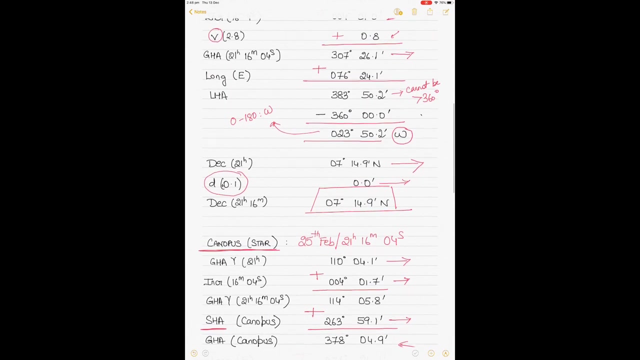 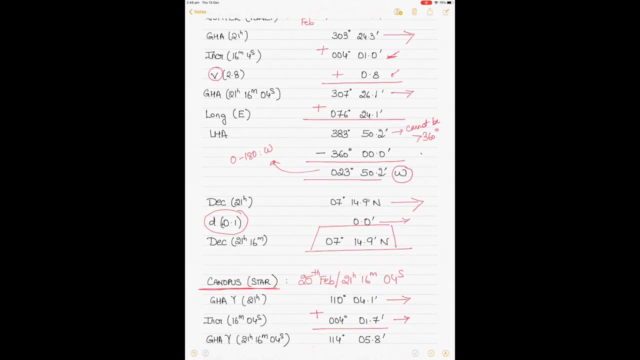 angle between, angle between the greenwich meridian and the celestial body right now, in this case here, uh, well, here the gh is more than 360, so i will not use this example here. i'll use the example from. well, here, 307 degrees is the gha. so let let me, let me take this example here of the planet. 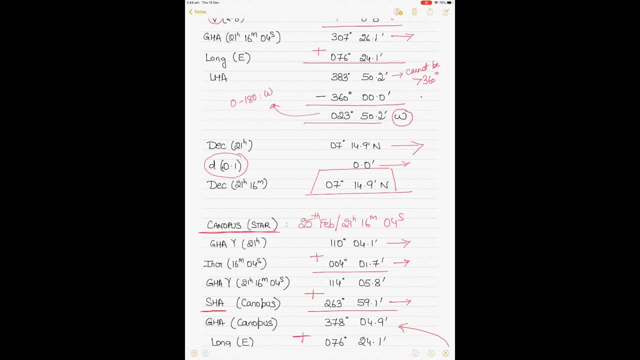 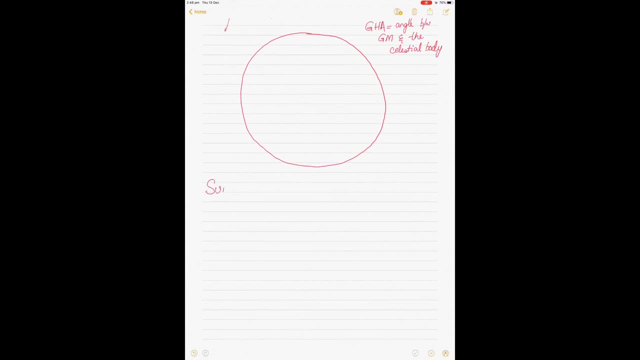 and here what we have done is basically let me write down the values of the. oh, let me take the first value itself. okay, sorry for all this confusion. so for the, the sun, that we calculated, let me write down here what we did. so the gha corrected gh-a value for. 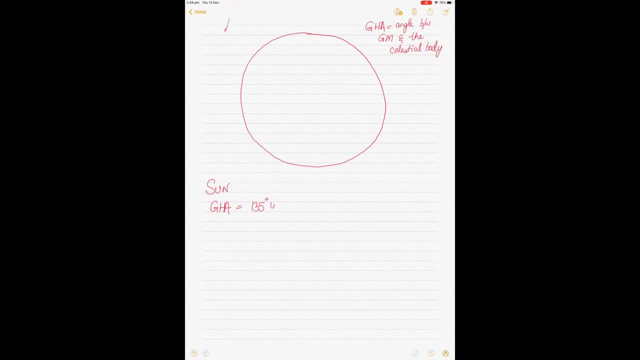 the sun from the first example was 135 degrees in 44.6 minutes. the lha value was 2 1, 2 degrees, 8.7 minutes, and the longitude was, of course, 76 degrees, 24.1 minutes east right, and the lha was, of course, east as well because it was more than 26 degrees, so it was比較海滩. 24.1 minutes east and the rha was of course east as well because it was more than 3, 3, 8. That is compared to the daily minute value because of course it was length, 2.01 per minuteô the room temp Fischercom. our table also has a Engendera. 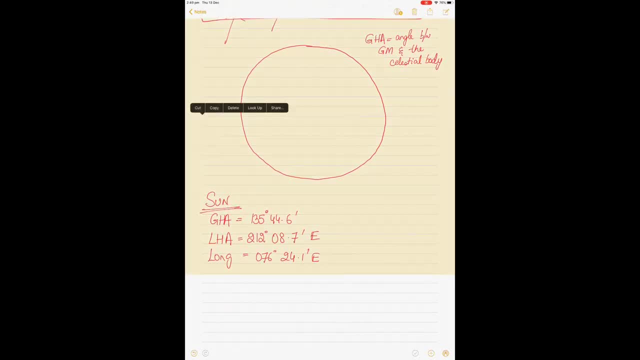 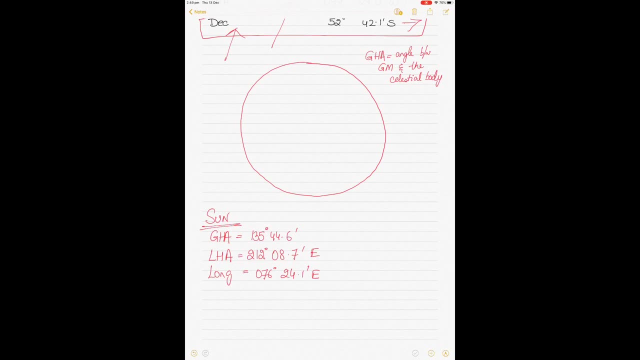 more than 180 now. this was from the Sun's example right now, if I need to conceptually visualize it, sorry, if I need to conceptually visualize it, G, H is the angle between the green which made in and the celestial body and it is measured westwards, Western, all right from the green which measured westerly. 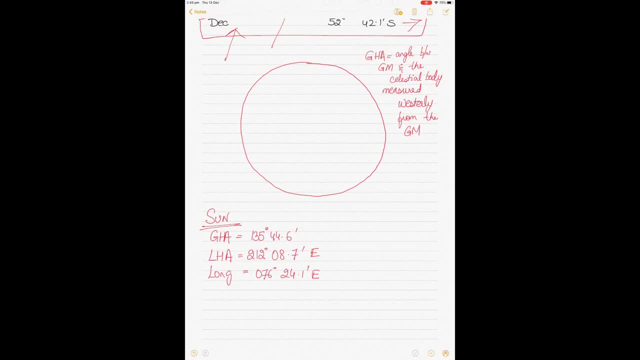 from the green which medium. well, so if I imagine this to be the green which medium, and if I go westerly and measured 135, it will be somewhere here with the celestial body and I'll draw a Sun here. if I measure this angle westerly, this 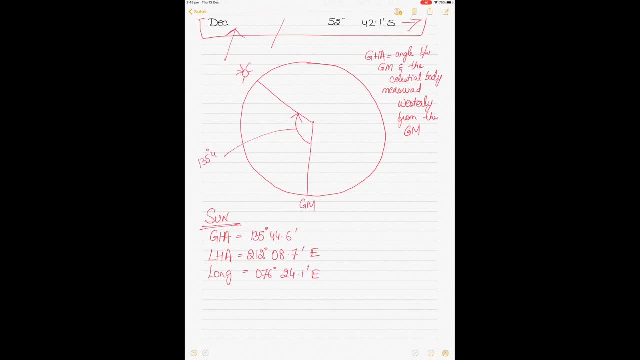 value here is 135 degrees. that's your GTA 44.6, right? that's how your Unbelievable looks. now, if you need to know what is LHA? no, silver energy is now the angle between the celestial body and the observer on the celestial medium, so the 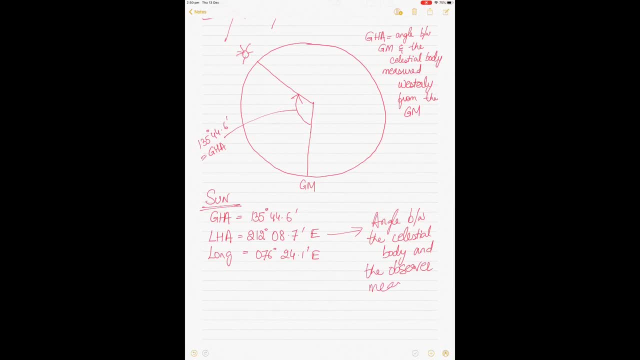 observer is you on the ship, right, and this is also measured Western, but from the celestial body. so let's hear: LHS: 2, 1, 2 degrees, 8.7 minutes. so what I will do is I will measure 2 1, 2 from here. so if this is 180, I have got another 45 to. 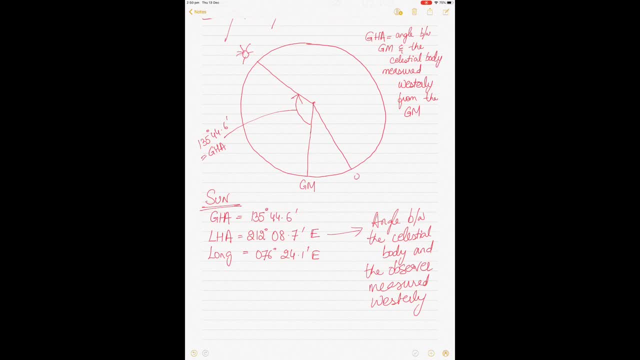 somewhere, somewhere here, becomes your body. but it's you on the ship, the celestial observer right. so this measured here westerly is the LHA and you can see here. in this case your longitude is 76 degrees 24.1 minutes East. so you can see, the longitude is actually the angle between. 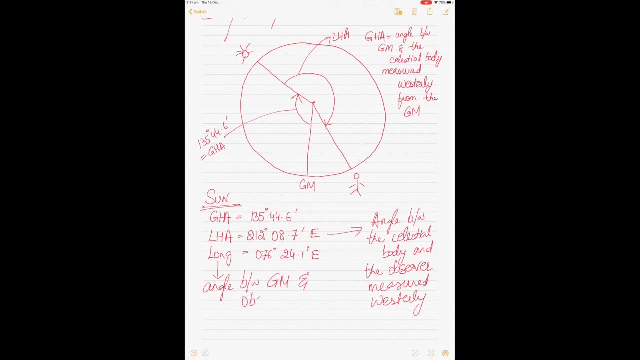 you can see here, in this case your longitude is 76 degrees 24.1 minutes East. so you can see, the longitude is actually the angle between greenwich meridian and the observer, and this is measured westerly or easterly depending on whether you are on the east or the west of the greenwich meridian. 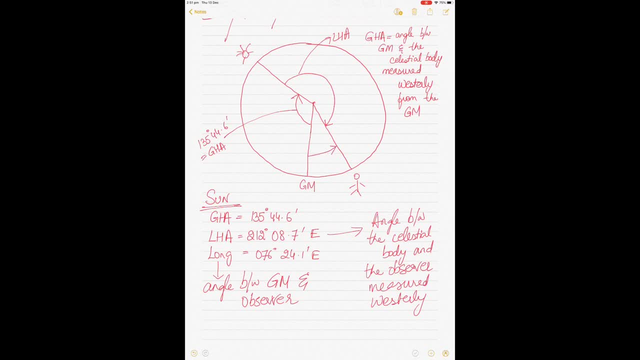 you can see, here, in this case, you are on the east of the meridian right, and that is why this is the relationship between, and that's why your longitude here is 76 degrees 24.1. and if you viewed the other way around, if I had drawn the longitude, 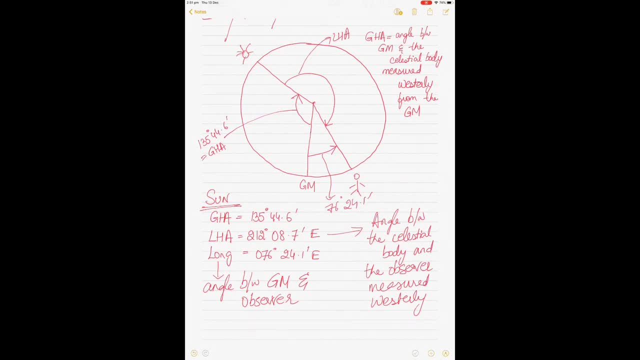 earlier, you would know why the body is up there, why the LHA is up there and why the LHA is east. so you get the concept or the idea between LHA, the longitude and the GHA right. so go through this video again. I will make some more videos on theories regarding LHA, GHA, longitude. 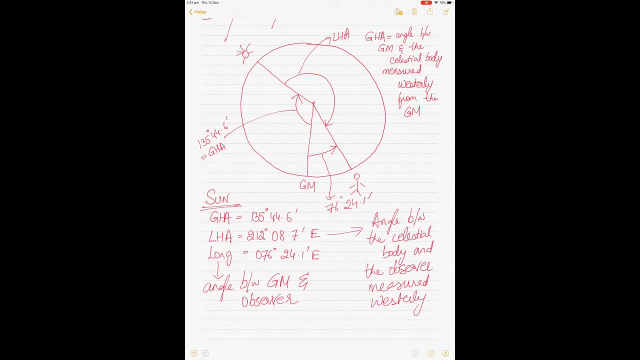 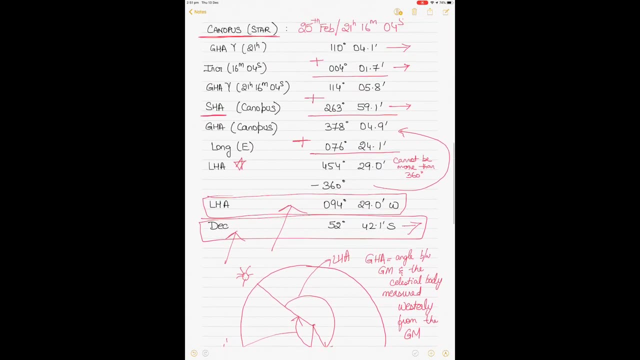 so if you found this a bit confusing, don't be disheartened. I will put up more videos, more theory and but right now I was focusing more on the calculations. so go through these videos and, multiple times, see the corrections that we applied to the planets, to the stars, to the planets, and so on and so forth. so 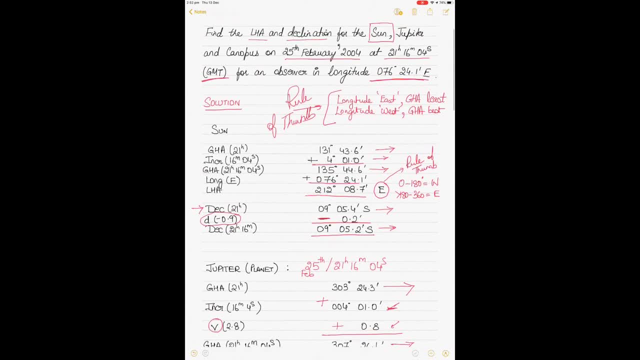 go through these videos and, multiple times, see the corrections that we applied to the planets, to the stars and to the Sun, and how did we get the LHN declination. that's more important. remember the rule of the terms that we used and the concepts that we used to get it all right. so I'll catch you soon. with. 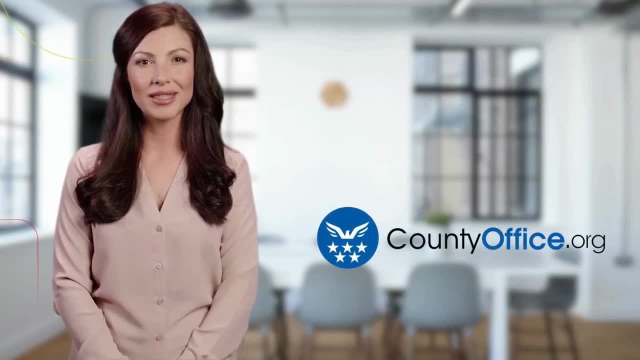 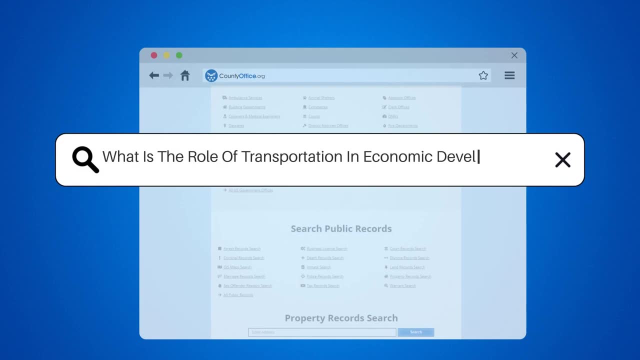 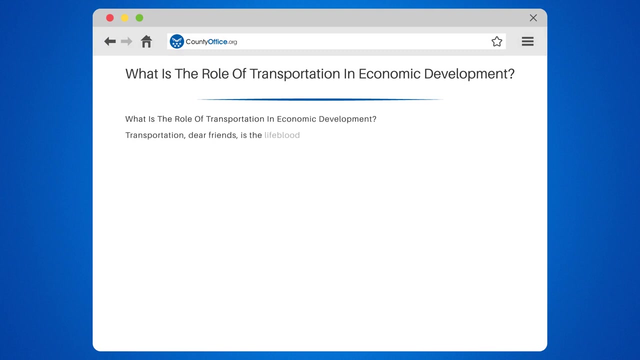 Welcome to County Office, your ultimate guide to local government services and public records. Let's get started. What is the role of transportation in economic development? Transportation, dear friends, is the lifeblood of any economy. It's like the circulatory system. 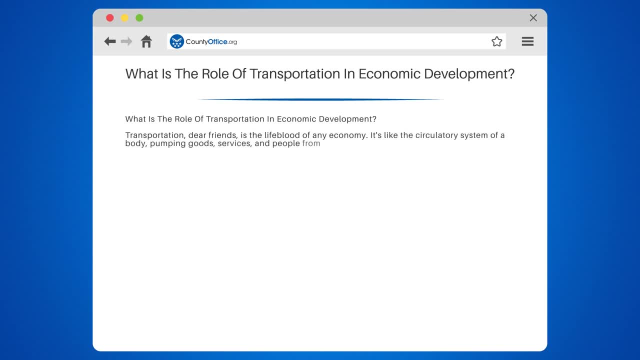 of a body pumping goods, services and people from one place to another. Without it, economies would be like bodies without blood flow, stagnant and unproductive. Transportation infrastructure such as roads, bridges, airports and ports plays a pivotal role in connecting different regions. 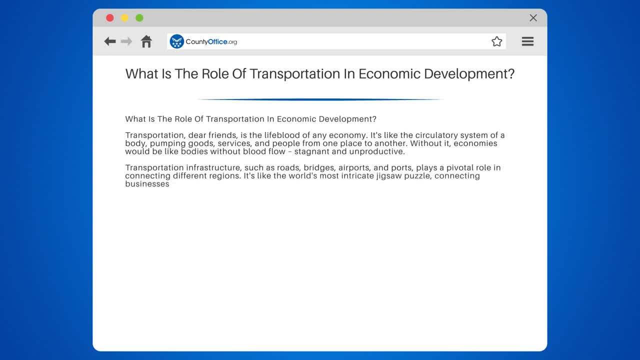 It's like the world's most intricate jigsaw puzzle connecting businesses with customers, suppliers with manufacturers and people with jobs. When transportation is efficient, it reduces the cost of moving goods and people. It's like having a discount coupon for every journey, making trade more profitable and boosting economic growth. 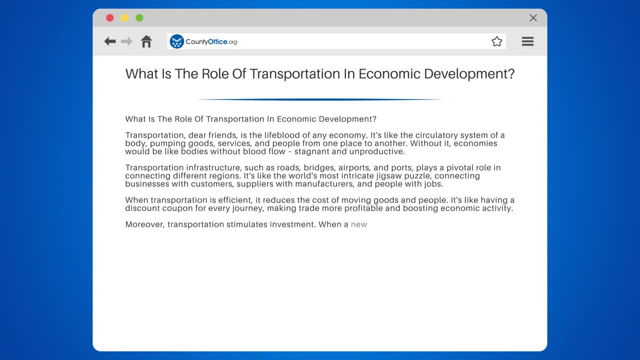 Moreover, transportation stimulates investment. When a new highway or airport is built, businesses often spring up around it like mushrooms after a rain. This leads to job creation and increased economic activity. But hold on to your hats, because transportation doesn't just move goods and people, It also moves ideas. By connecting different regions, it allows 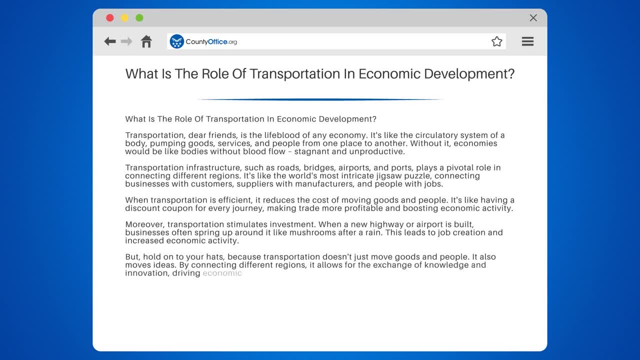 for the exchange of knowledge and innovation, driving economic growth. So, in a nutshell, transportation is a way of moving goods and people. It's like the world's most intricate jigsaw puzzle connecting businesses with customers and people with jobs. It's like the world's most intricate jigsaw puzzle. making trade more profitable and boosting economic growth. So, in a nutshell, transportation is a way of moving goods and people. It's like the world's most intricate jigsaw puzzle connecting businesses with customers and people with jobs. It's like the world's most intricate jigsaw puzzle. 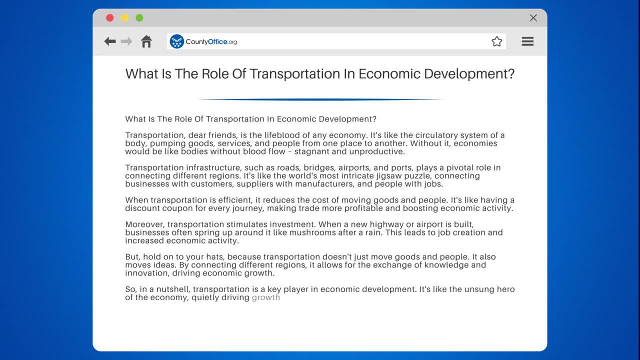 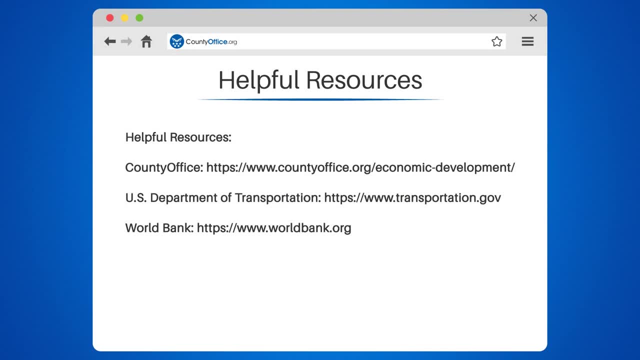 keer ev dungeon is a key player in economic development. It's like the unsung hero of the economy, quietly 과� Bangalore. growth, emin running prosperity. To learn more, check out these links, which you can click in the description below.